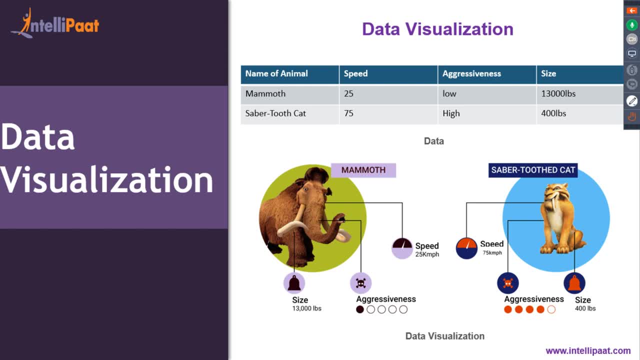 on a huge data set which comprise of around thousand columns and one million rows. Now finding insights from this data is extremely hard. So this is where we can take the help of data visualization to find interesting patterns from the data. So we have this data set over here. 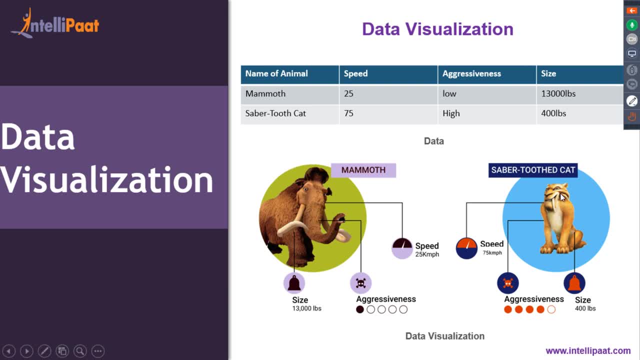 and this data set is represented in the form of images. Now we see that these images help us to easily identify the features of these animals. So we've got mammoth over here and with the help of this image, we can see that the size of mammoth is. 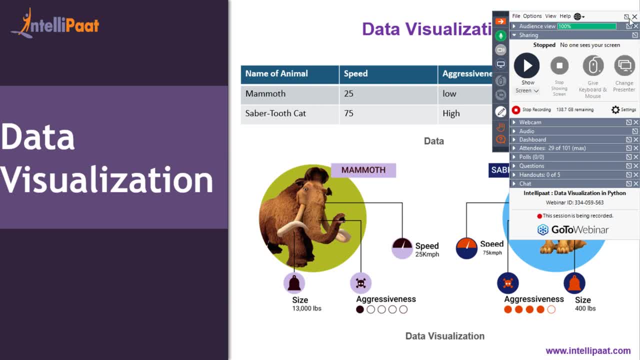 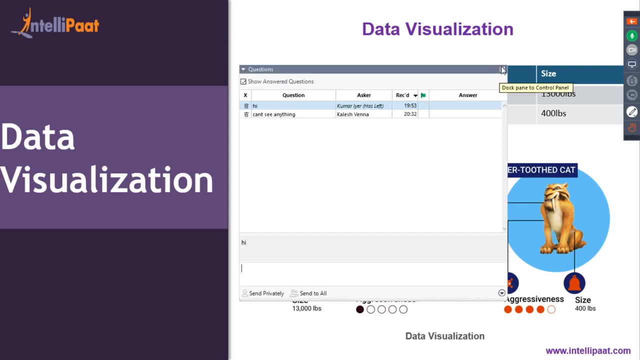 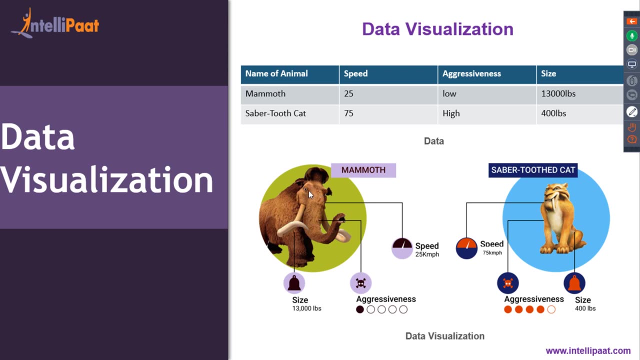 right. So sorry for that interruption. So, as I was saying, we've got these images over here and these images easily help us to identify the features of these animals. So this is mammoth, and this represents the first record. and this is saber tooth cat, which represents the second record. And with the help of this image, we can see that the size of mammoth is. 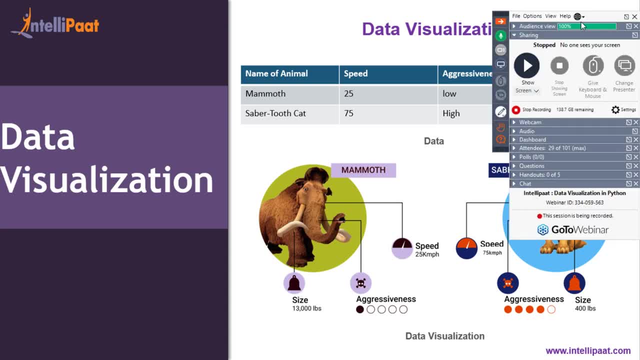 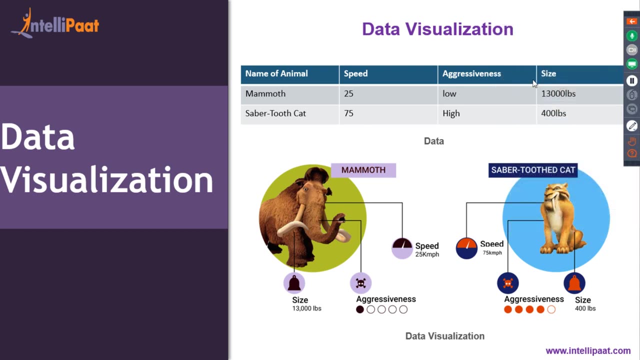 really not enough. Yeah, sorry, So there seems to be some technical issue with the screen, So now I hope that the screen is visible to everyone. Alright, so let me actually start from the beginning was saying: data visualization is basically the art of representing raw data in the form of beautiful 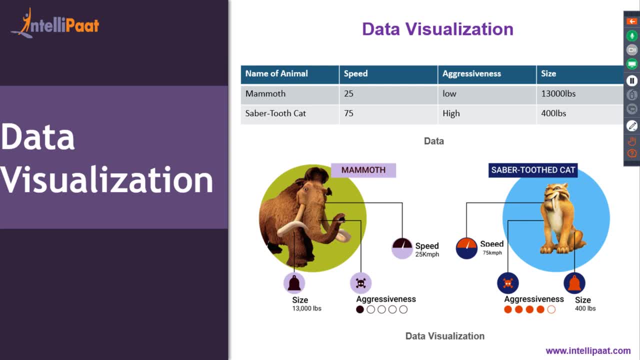 and aesthetic graphs. now let's take this example where you're working on a huge data set which comprises of around thousand columns and one million rows. now, to find insights from this extremely huge data, it's very, very difficult. so this is where we can take the help of data. 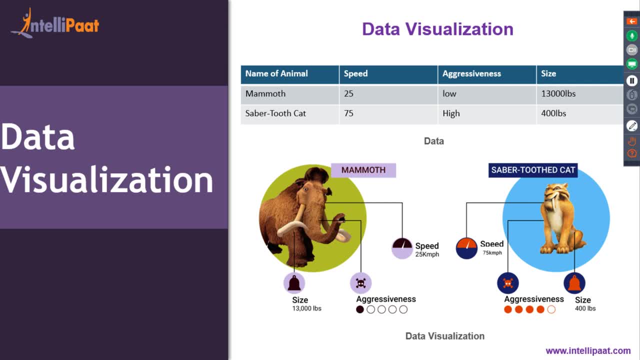 visualization to find extremely meaningful insights from the data. so over here we've got this data set and we have represented this data set in the form of these images. so this is the image of mammoth, which represents the first record, and this is the image of saber-toothed cat, which represents the 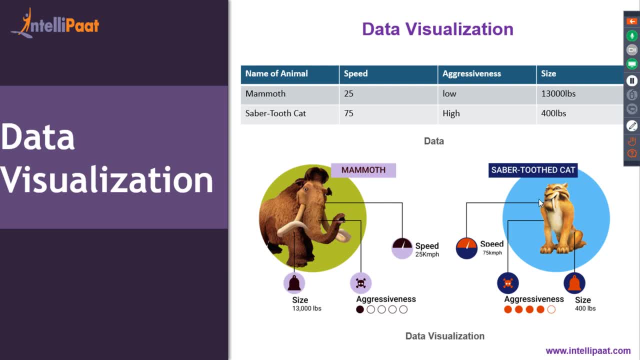 second record and we can easily find insights of these two animals from this image. so we see that the size of mammoth is 13 000 lbs and its aggressiveness is very low and the speed of mammoth is around 25 kilometers per hour. and then we've got saber-toothed cat. so we see that from. 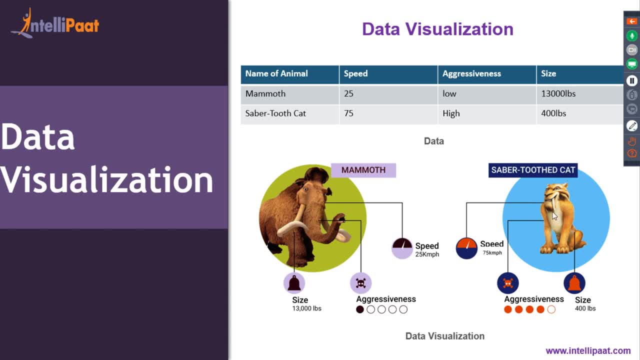 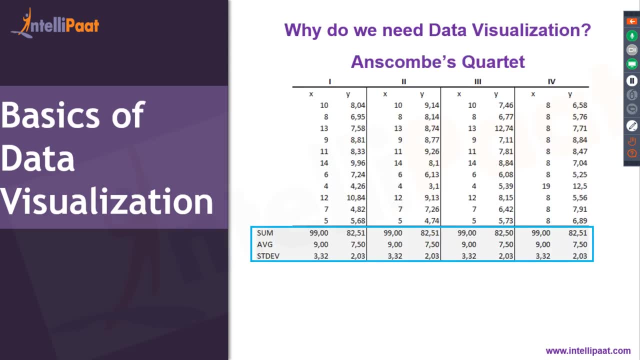 this image, the speed of saber-toothed cat is 75 kilometers per hour, its aggressiveness is very high and its size is 400 lbps. right, so now again, let's take this example. so we've got this anscombe squatted. so this data set basically comprises of four files in total, and these four files have: 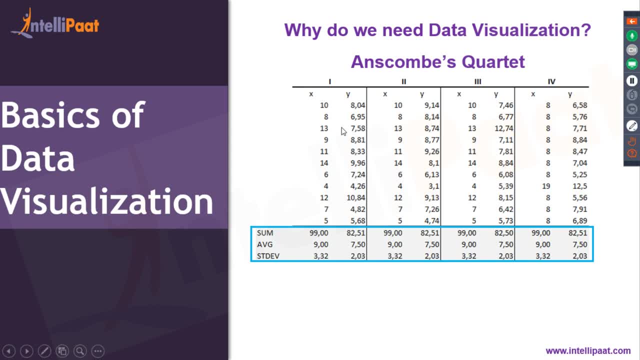 these values of x and y. now, if you look closely at this data set, you'd see that these values are very similar to each other. now let's actually go ahead and find the sum, average and standard deviation for x and y for all of these four files. now, again, if we look at, 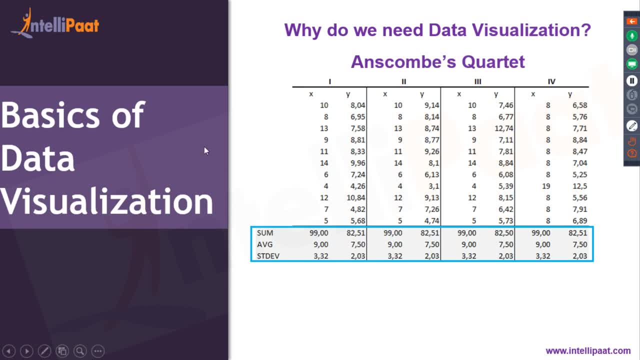 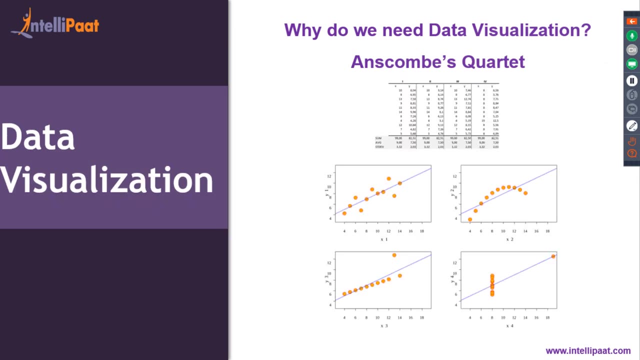 this result, we see that the values of x and y are same throughout all of these four files. so if we just have a glance at some average and standard deviation, then we might think that the x and y values for all of these four files are very similar. but let's actually go ahead and 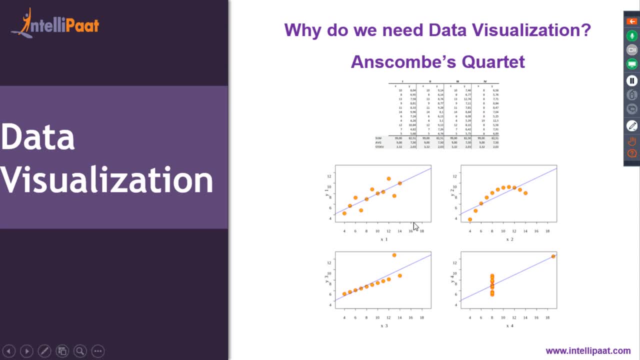 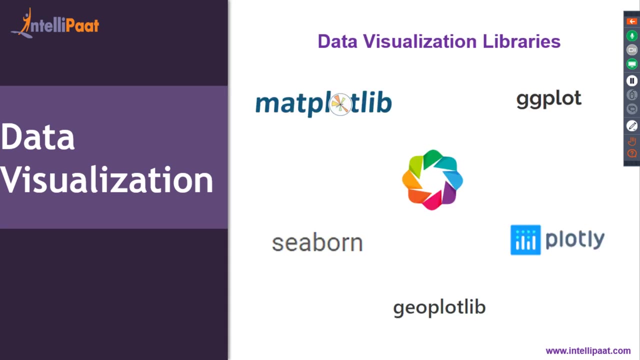 plot these four files. so when we actually make a pictorial representation of this data set, we see that the relationship between x and y is very different for these four files, and we were able to understand this with the help of data visualization. so now that we know the importance, 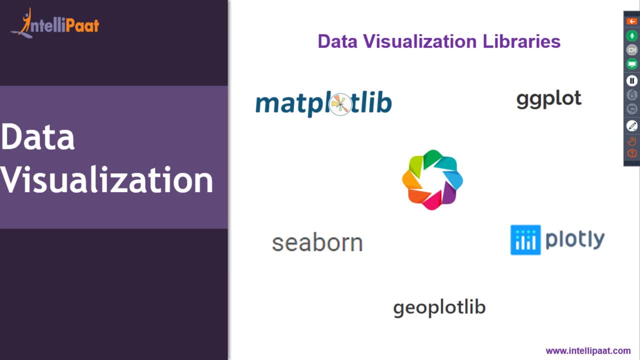 of data visualization. let's actually look at the different visualization libraries with python provides. so python has got matplotlib, ggplot, plot, legio, plotlib and seaborn, and in this session we're going to do data visualization with the matplotlib package. so let's go to jupyter notebook. 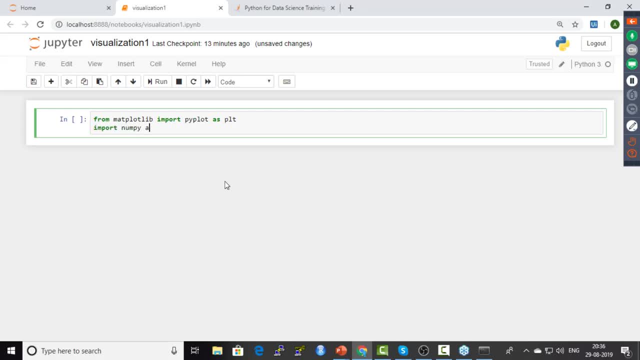 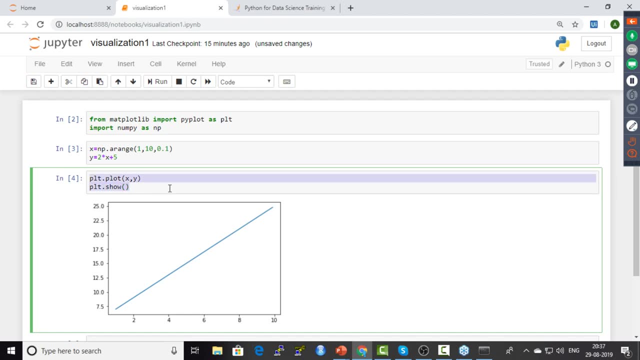 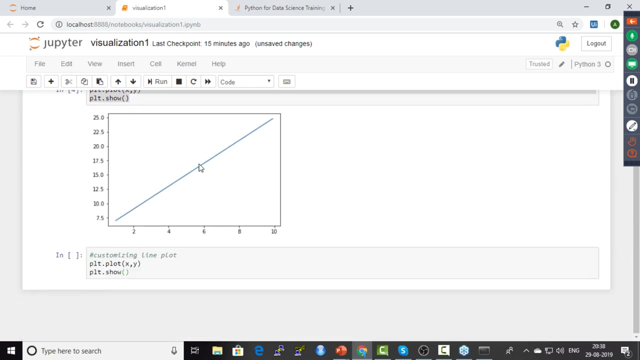 i'll also import the numpy package, so i'll type in import numpy as np, right, right? so i'll just copy these two values over here and paste them over here. let me also copy these two lines over here, right? so now what i'll do is i will actually um, add some colors to this line plot, so i've 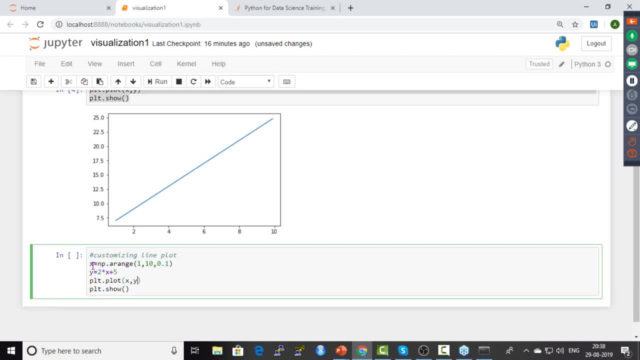 got the value for x, i've got the value for y, for all of these x and y values, so i'm just gonna go ahead and create a model and then i'll just select all of these files that i want to easiest the value for y. now what i'll do is i will change the color of this, so i will use the attribute. 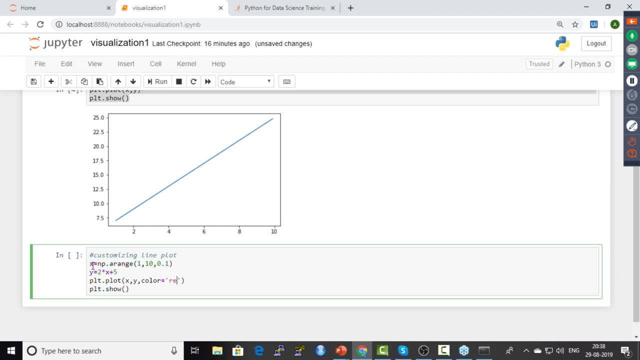 c-o-l-o-r and i'll give in the color. let's say red to this. and after this, what i'll do is i'll assign a title to the plot. so for that i'd have to use plt dot title and the title which i'll be. 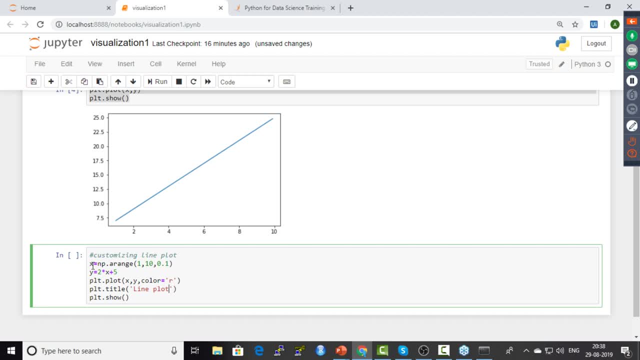 giving. this is line plot and i can also give labels to the x-axis as well as the y-axis. so to give labels to the x-axis i'd have to type in plt, dot, x label and i'll give in the x axis label as x axis. similarly, i haven't given the label for the y. 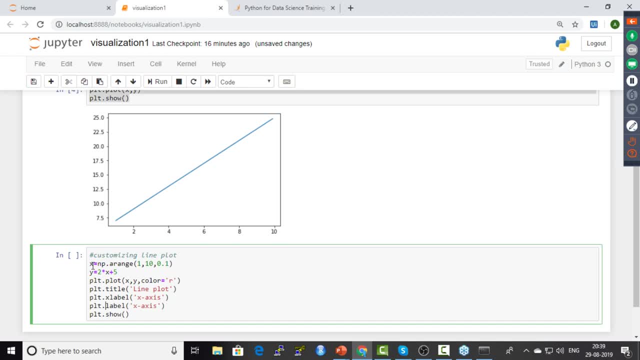 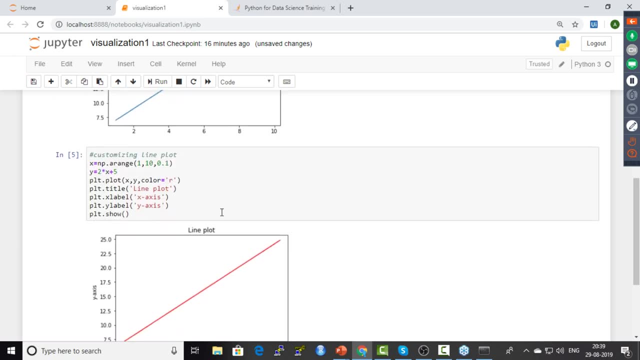 axis. so this would be plt dot y label and the label which i'm giving to the y-axis is y-axis. as simple as that, right? so we have customized a line plot. so we started off by creating a simple line plot where the color of the line was blue. after that we made a line plot, and this time 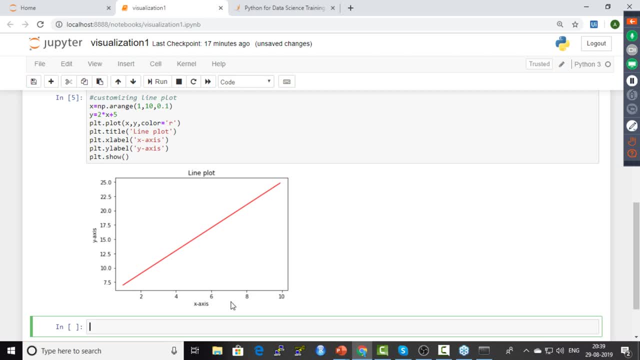 we've customized the line plot, so the color of the line is red, and we've also assigned the labels for the title for the x-axis and also for the y-axis. now we'll see how to do a bit of subplotting, that is, we'll see how to add two plots in the same figure, right. so for this, what i'll do is i will 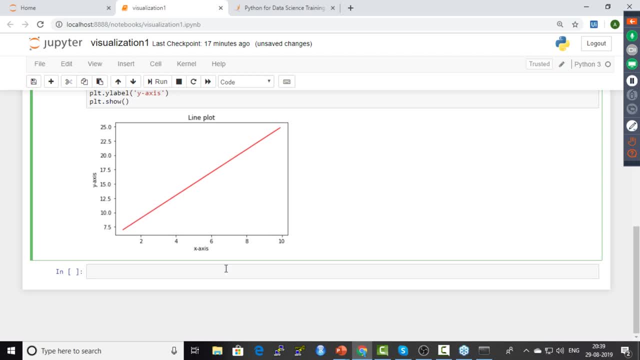 actually have two y values. so let me copy this and let me paste it over here, so the x-axis values would be the same and i'll have y1 over here. so y1 is 2 cross x plus 5. then i'll also have y2. so 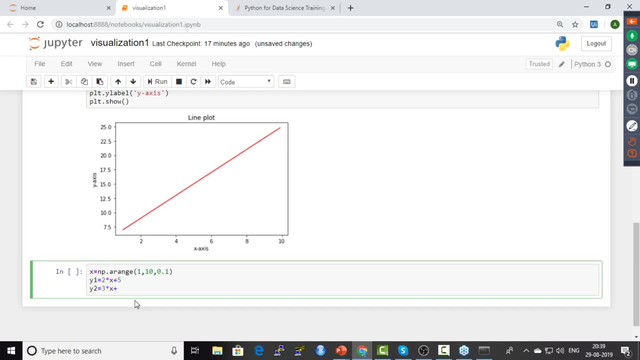 y2 would become 3, cross x plus 10, and with the help of these values i will create two plots. so to have two subplots in the same figure i would have to use pltsubplot method, and this basically takes in three praise parameters. so the first parameter is the number of images in the rows and number of images in. 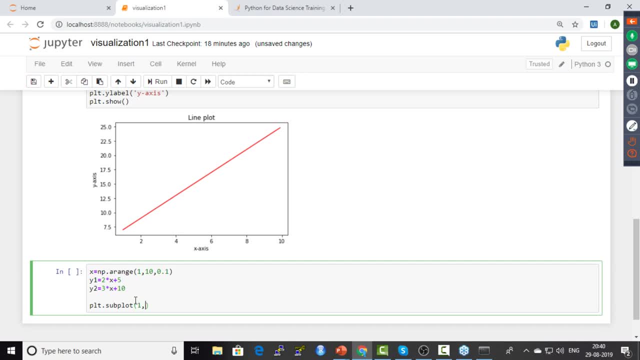 the columns. so since i want two images, this would basically mean one comma two. so i'll have one row and two columns and i'll put in one over here. so this one basically means that i am activating the first subplot. now let me go ahead and plot this. so plt, dot, plot and the values would be: 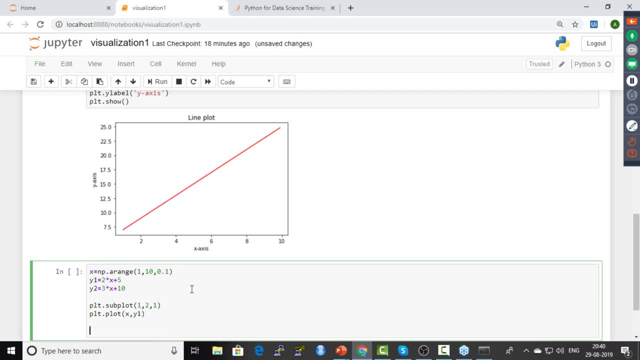 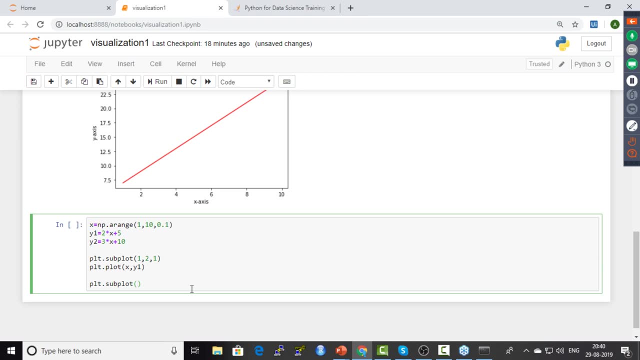 x, comma y1. now let me go ahead and also add the second subplot. so this time it will be plt, dot subplot and i'll give in those three parameters. so one comma, two, so one row, two columns, and this time i'll activate the second subplot, so i'll add in two over here. now let me copy this: 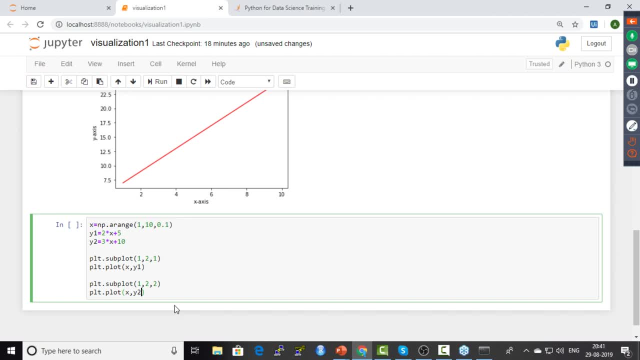 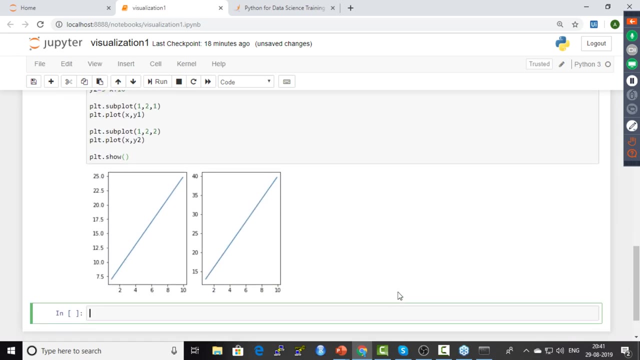 paste it over here and i'll plot the second graph. so this time it is x comma y2, and i'll finally show the figure. so plt dot show. now let me click on run right. so now we have created two plots or two subplots in the 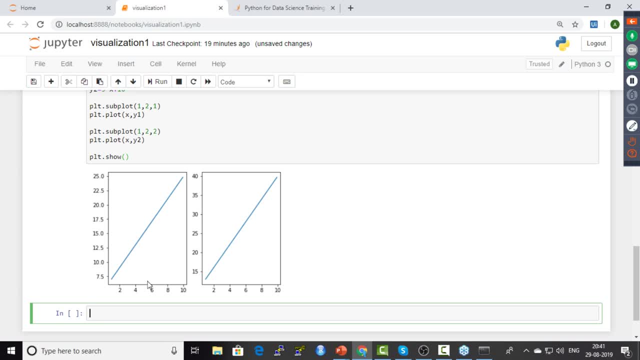 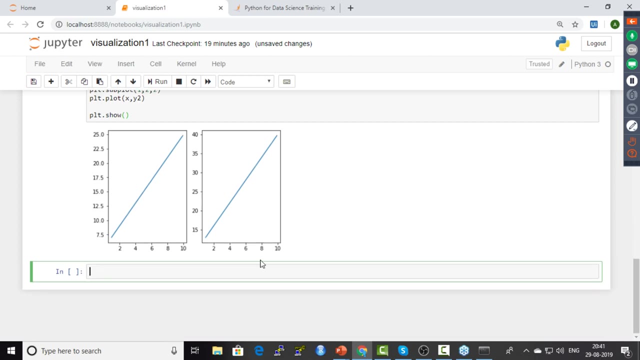 same figure and if you look at these values, these values are different, right? so the x-axis values are same, but y1 and y2 are different. so, over here, y1 ranges from 5 to 25 and y2 would range from around 7.5 to 40, right? so this was line plot. now let's go ahead and see how to create a bar plot. 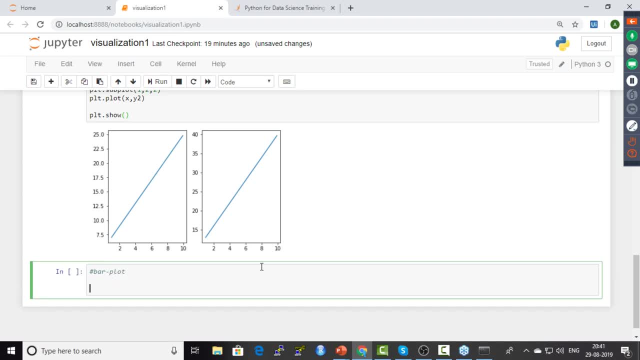 so let me just type in bar plot over here now. to create this bar plot, let us first create the data set. so i'll go ahead and create a dictionary first and i'll name that dictionary as fruit. so to create a dictionary we'd have to, given these curly braces. so we have a key value pair. 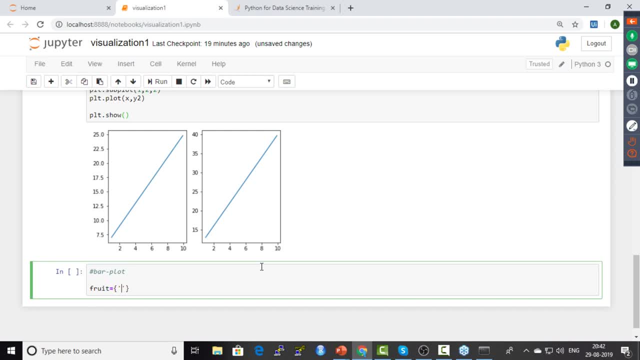 in a dictionary. now let me assign the first key value pair. so let's say: my first fruit is apple and there are 30 apples. the second fruit is mango and there are 45 mangoes. after that I've got banana and I've got around 10 bananas. now I will add. so now what I'll do is I'll extract the individual. 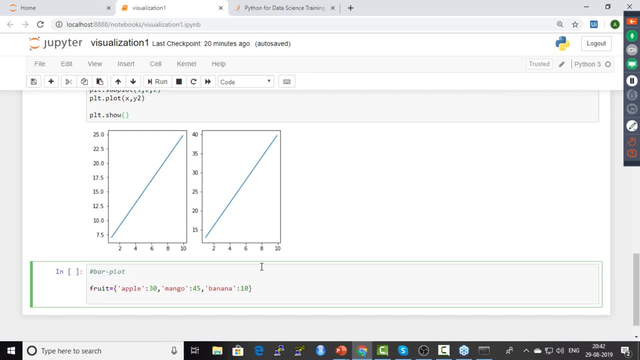 keys and individual values and store them in separate objects. so over here I will create a new object and name that object as names and I'll extract only the keys from this dictionary. so I'd have to type fruit dot keys and I'll store the keys and names. similarly, I'll extract the values, so I'll store the. 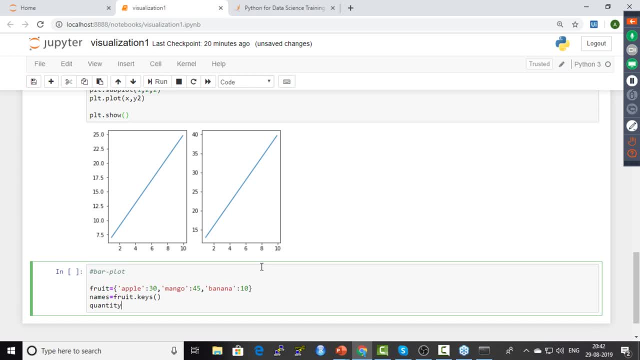 values and quantity. so I'll have to type in fruit dot values, right? so I've extracted the keys, I've extracted the values. now I'd also have to store this in the form of a list. so let me just type in list and let me go to the list, and let me go to the list and let me go to the list and let me. 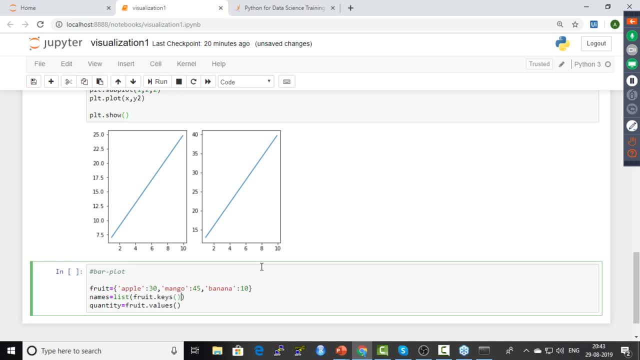 cut this and let me piece this inside a list. similarly, I do the same thing over here. I'll type in list: let me cut this from over here and let me piece this inside the list. right, so we had created the dictionary. now let me just print out. 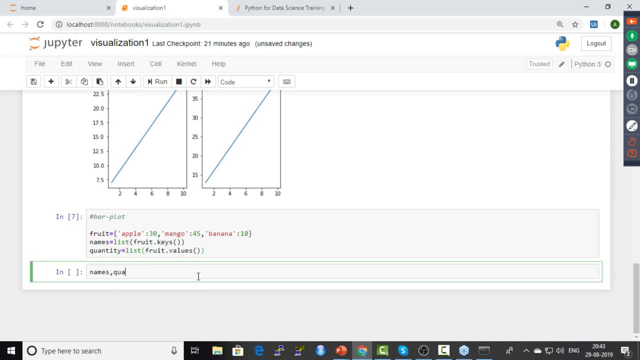 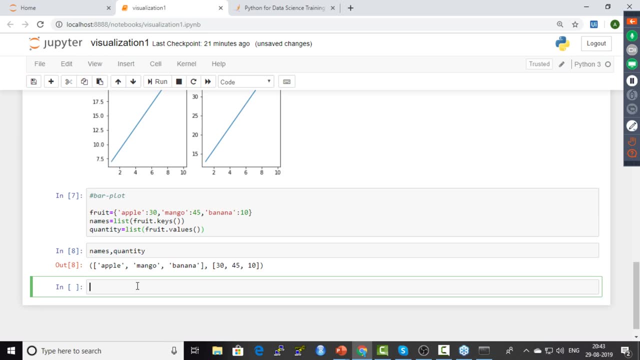 names and quantity over here. names, quantity, right. so we've got the individual names of the fruits and the quantity of the fruits over here. now we'll go ahead and create this bar plot. so to create the bar plot we'll have to type in PLT, dot, bar and. 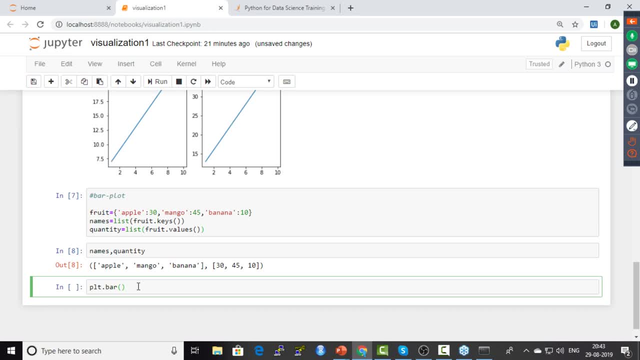 this basically takes in two parameters. so the first parameter would be the names of the fruits, or the categorical variable which contains the names, and then we'll have the values. so values, I have it in quantity now. after this I'll just show this. so PLT dot show. 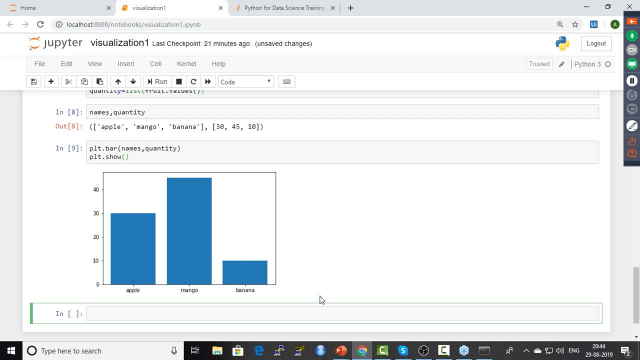 right. so we have successfully created this bar plot where we have the names of the fruits on the x-axis and the quantity of the fruits on the y-axis. so again, this plot easily helps us to understand that the major quantity of the fruits belongs to mangoes and the minimal quantity of the fruits it belongs. 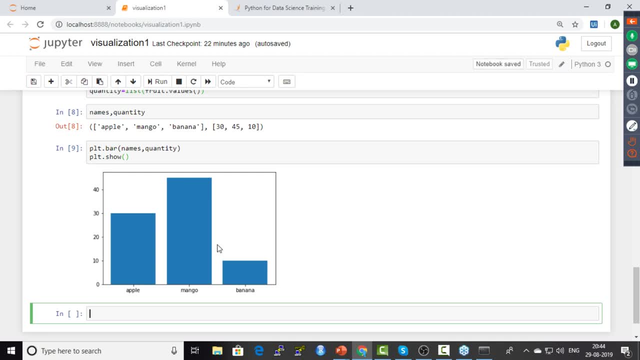 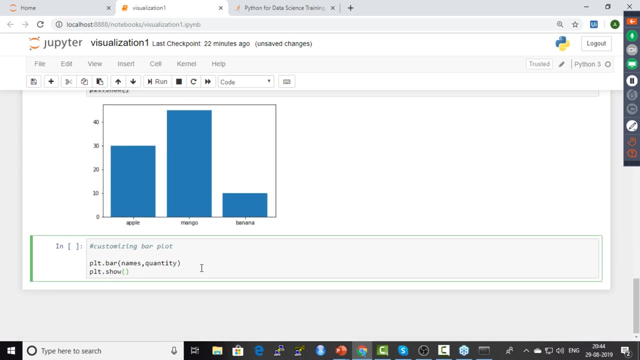 to bananas. now let's actually go ahead and also customize this bar plot. so I'll just type in customizing bar plot and I'll copy this same thing over here. Now let me add a title, x-axis label and y-axis label, So plttitle, and I'll assign the title to be, let's say, distribution of fruits. 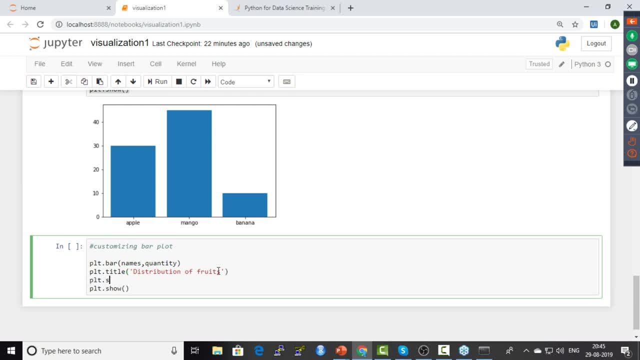 And then I'll give the x-axis label, So pltxlabel And the x-axis label would be fruits Of that. I'll give in the y-axis label, So it'll be pltylabel And this label would be quantity. 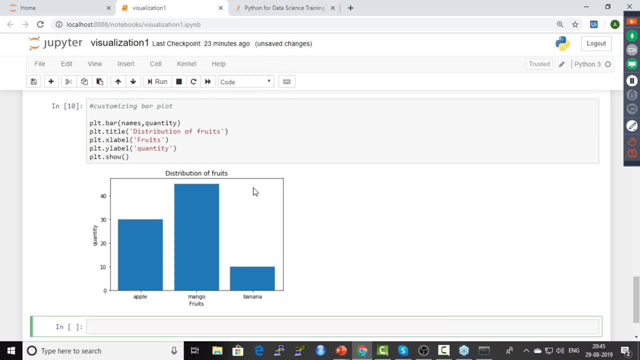 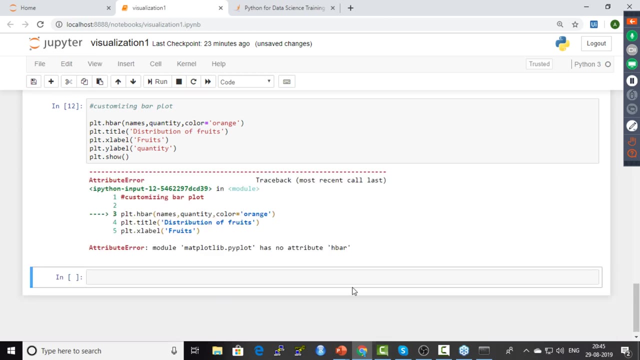 Right Now, let me print this out, Right? So we've added the title, We've added the x-axis label, So I added the y-axis label And let me use the argument color And I'll, let's say, give in the orange edge bar, Right? So let me actually change this first. 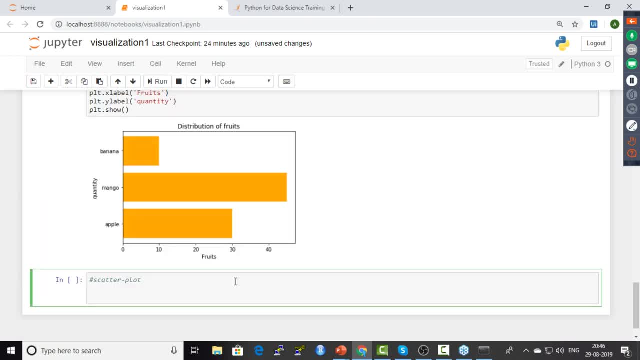 pltbar. So we've got this. Let's start off by creating the data for the scatterplot. So what I'll do is I'll have my first data and I'll add in some values over here, So 10,, 20,, 30,. 40,, 50,, 60, 70. So there is a lot of data, So I'll add in some values over here. So there is a lot of data, So I'll add in some values over here. So there is a lot of data. 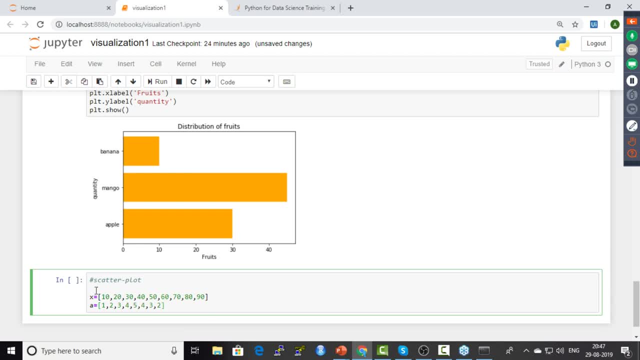 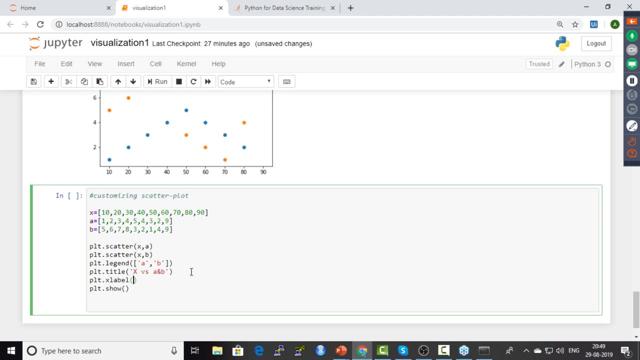 So there is a relationship between x and a And there, all that, the number of points are same. Let me add the x-axis label again, So it'll be the same pltxlabel And it'll just be x. Now. 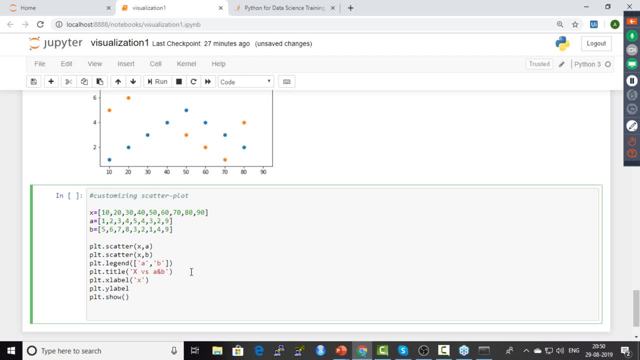 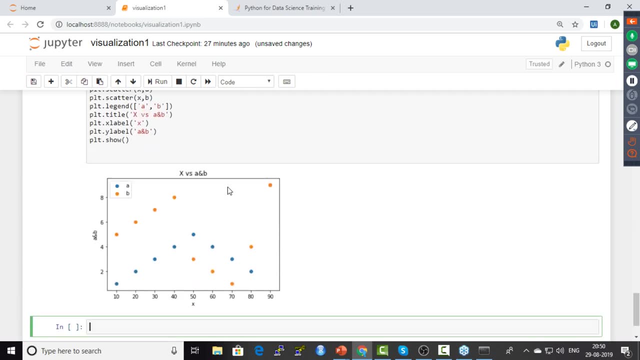 let me add the y-label, So pltylabel. So this would be a and b. Now let me print this out, Right? So we've got the title, We've got the x-axis label And we've got the y-axis label. 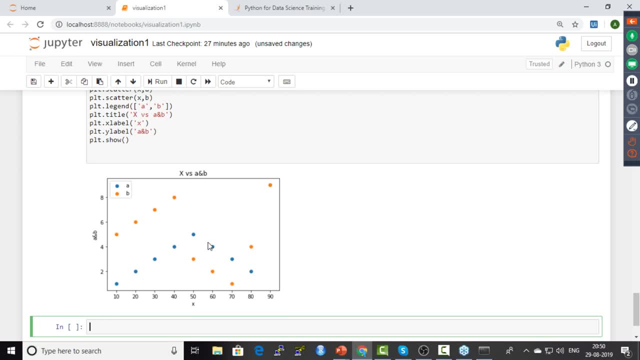 Now, what we'll do is we'll add in some values over here. So let me add in some values over here. Now, what we'll do is we'll change the size of these points, Right. So let's see how can we do. 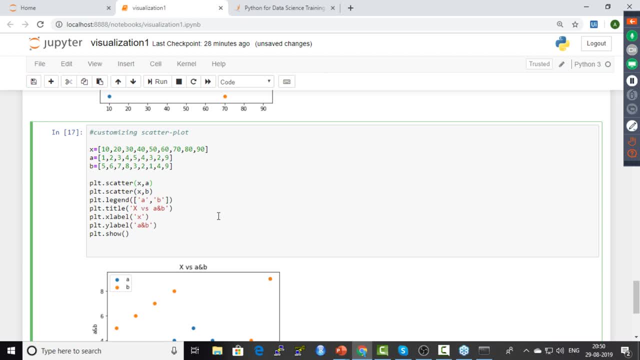 that. So to change the size of these points, we've got a parameter which is s, So this stands for the size. Now let me set this to be 200.. And let's see what happens. Right, So we see that the. 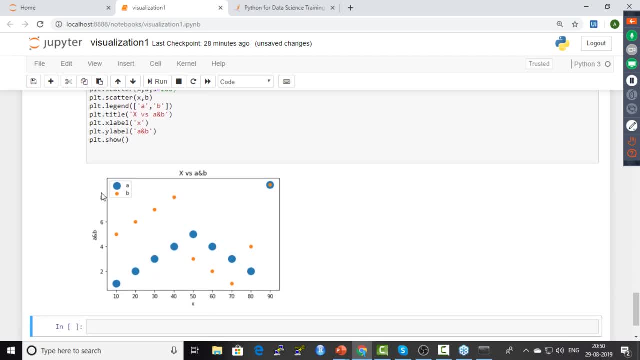 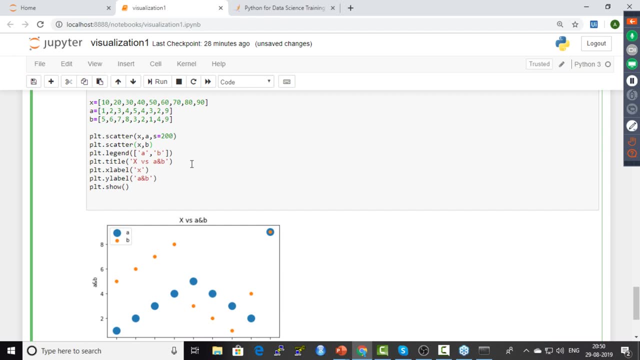 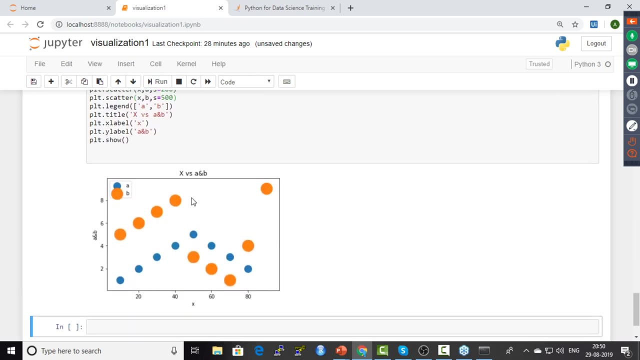 size of these points where the relationship between x and a has changed, Right, So this has changed to 200.. Now let's also change the size of these points, So I'll set this to be, let's say, s equals 500 over here, Right? So we've changed the sizes of both of these points. 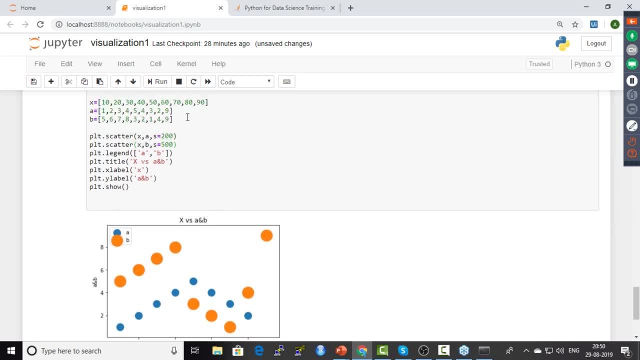 over here, And we can also change the shape of these points, Right, So I'll change the shape of this. So, over here, to change the shape, we have this argument called as marker And let me give in the value 3.. So if I give in the value 3, I have this over here Now. 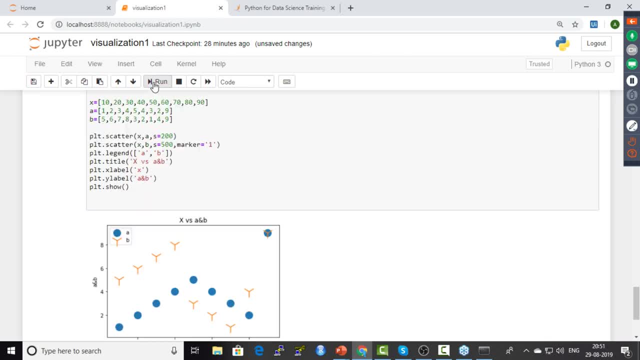 instead of 3,, let me put it to be 1.. And let's see what do we get Right. So over here this is tilted downwards. Now let me give in the value 2.. And let's see what do we get Right. So this time it is tilted. 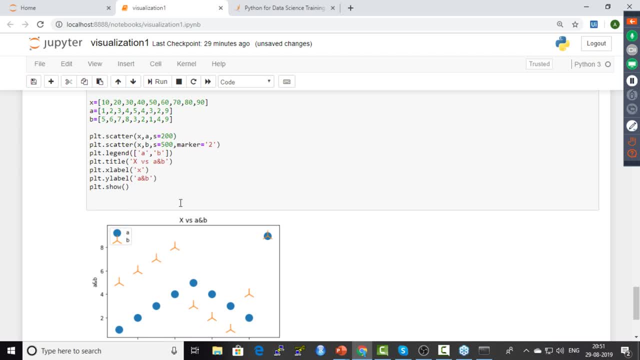 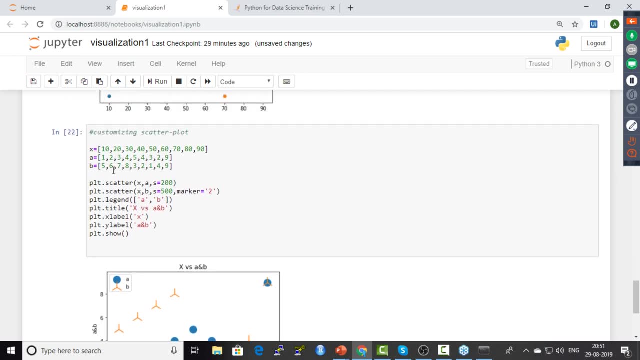 upwards Right, So we can have different markers or different shapes for these points over here Right And we can also change the size of this figure over here. To change the size of the figure, So above the plot method we would have to use in pltfigure. 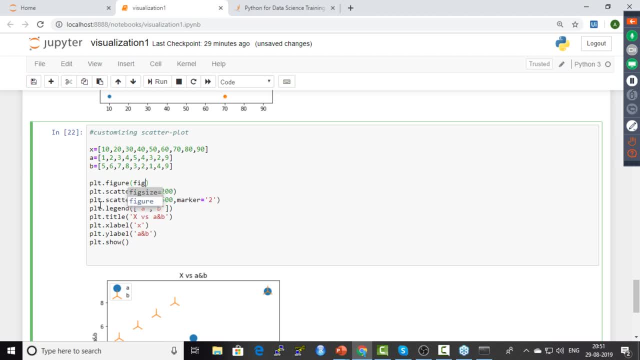 Let me just type in pltfigure And this takes in a parameter whose name is fig size, And I'll give it a tuple. So let me assign a value of 10,10 over here, Right. So over here I've increased. 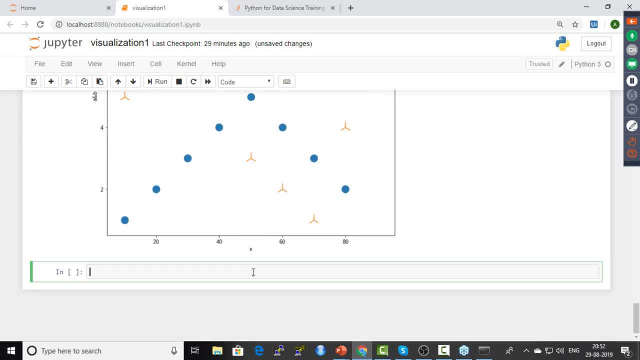 the size of this figure Right Now. after this, let me go ahead and start with the next geometry. So our next geometry would be a histogram. So let me give in the comment histogram over here. Now let me again create a list. So I'll give in different values for the list over here. So 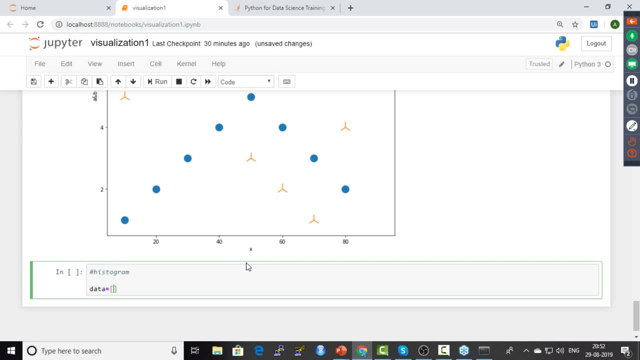 the numbers range from 0 to 9.. So I'll just give in 1,1,1.. And then let me just go ahead and keep on giving some random values between 0 and 9.. 7,, 5,, 4,, 3.. I'll again give a 1.. So I'm just making. 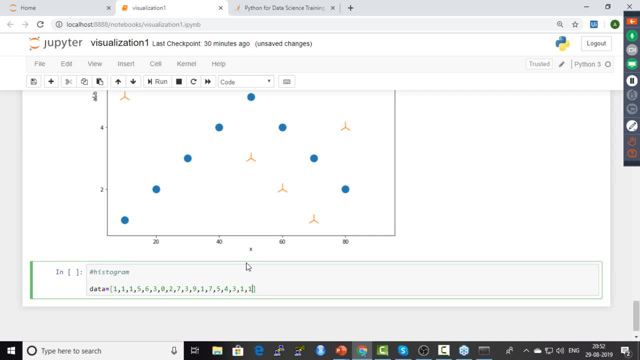 sure that there is a greater frequency of 1s over here, Right? So I'll just give a 1.. And then let me go ahead and give it a 2 over here, Right? So this is all of the data which would be going. 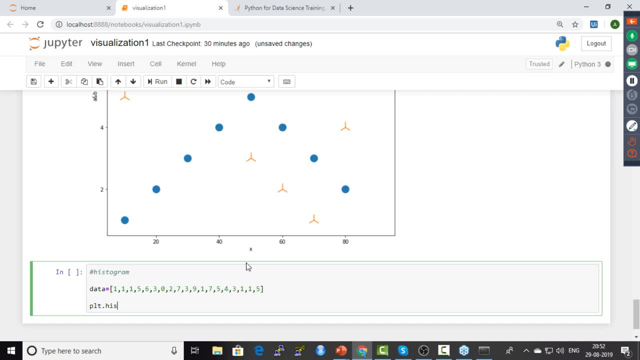 into the histogram. And to create a histogram I'd have to use PLT dot hist method And I will pass in the data inside this. Now to show the image I'll have to type in PLT dot- show. Let me. 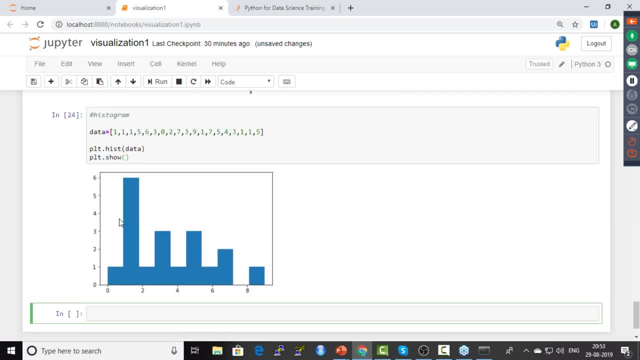 run this Right, So we have successfully created this histogram. So this basically gives us the distribution of this data And with the help of this, we can easily see that there is a greater ones in this data. and after that we've got three, we've got five right, so after one, the 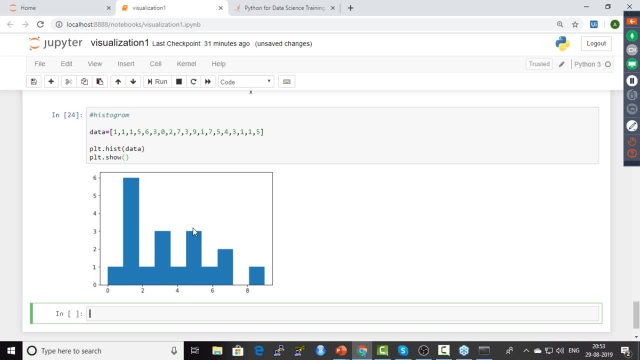 the frequency is high for three, and then there is frequency for five, right, and there is not even a single seven, or not even a single, sorry, there is not even a single eight over here, right? so that is what this gap tells you, right? so this is how you can interpret different insights from a 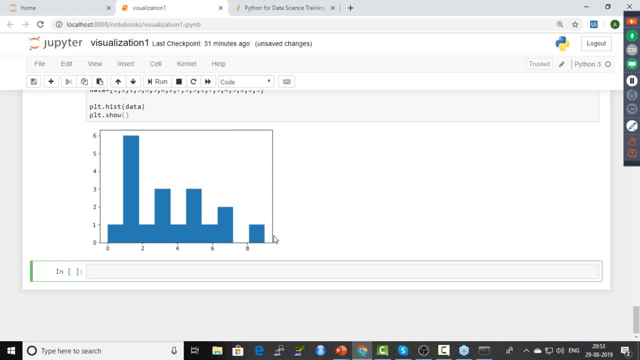 histogram. now again we'll see how can we create a histogram on top of a data set. so what i'll do is i'll go ahead and import the iris data set first. so for this i would require the pandas library, so i'll type in: import pandas as pd. now let me go ahead and load the iris data set, so i'll type in: 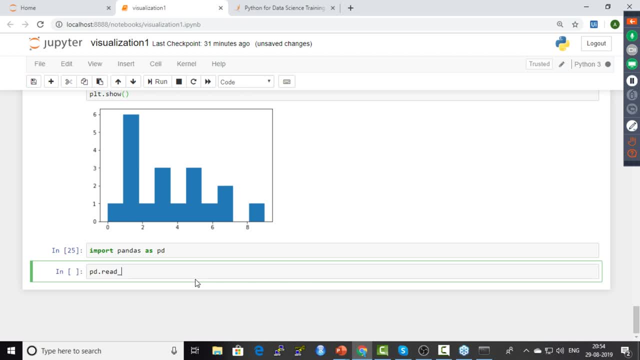 pdreadcsv. so, and let me give in the name of the file, which would be iriscsv, and i'll store this in a new object and i'll name that object to be iris. now let me have a glance at the head of this data set, that is, i'll have a glance at the first few records of this data set. so irishead. 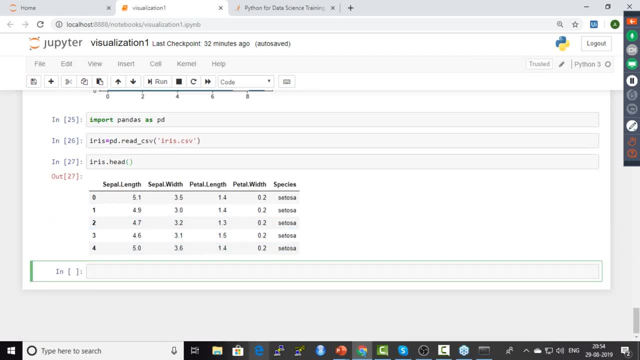 and this is our data set over here. now i want to have a- sorry, i want to make a histogram for this sepal length column from this iris data set. so all i have to do is i'll type in plt, dot, hist and i'll give in the data. so the data would be coming from this iris data set, so i'll 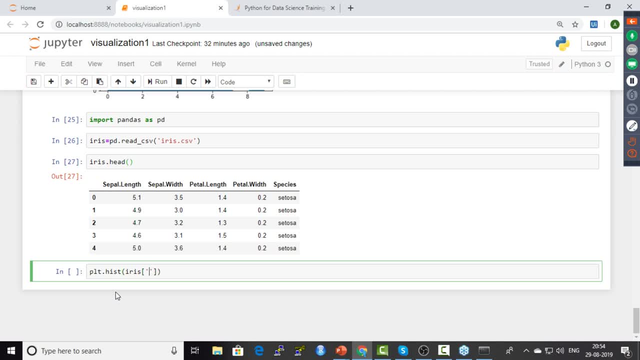 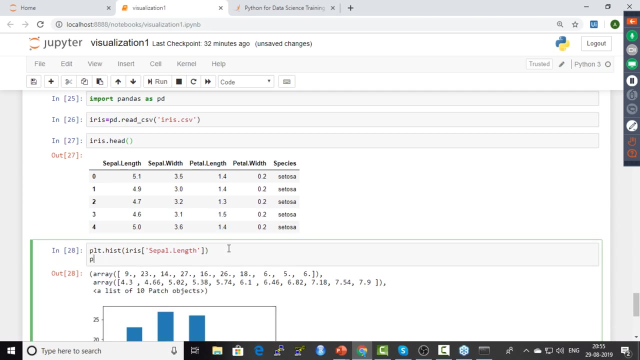 type in iris. i'll give in braces over here and let me select the column for which i'd want to make a histogram. so i'd want to make a histogram for this sepal length column. so i'll just type in sepal length. now let me run this. let me also just put in pltshow right. so we have successfully. 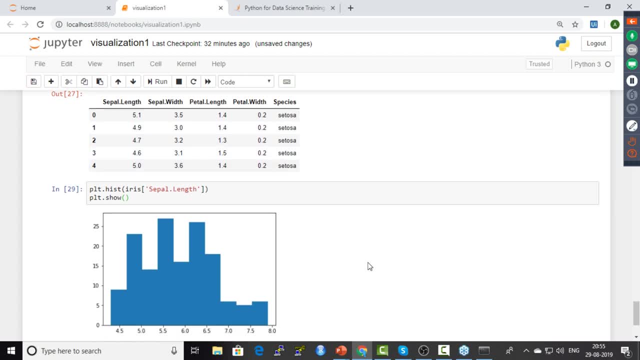 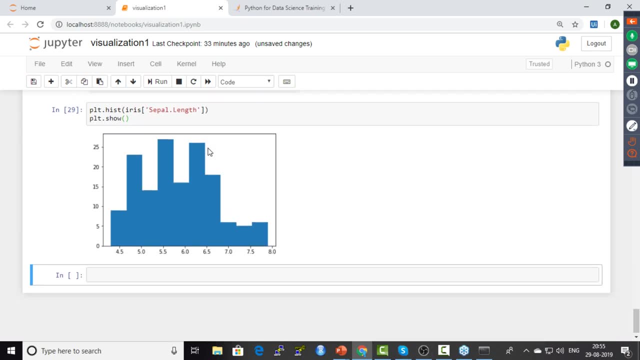 created a histogram for this sepal length column from this iris data set. so this basically tells us that when it comes to sepal length of the flower, so there is a greater frequency for the sepal length to be around 6.5 or 5.5, or you can see that the sepal length would vary mostly between 5 and 6.5. 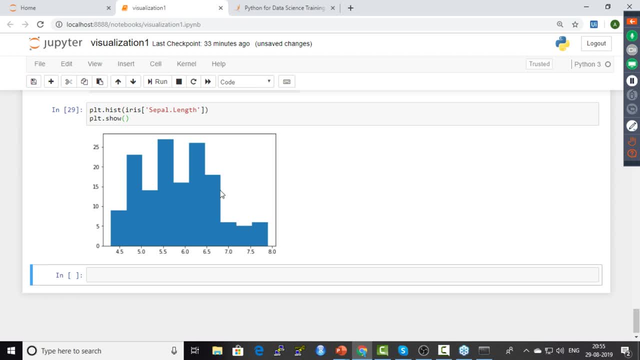 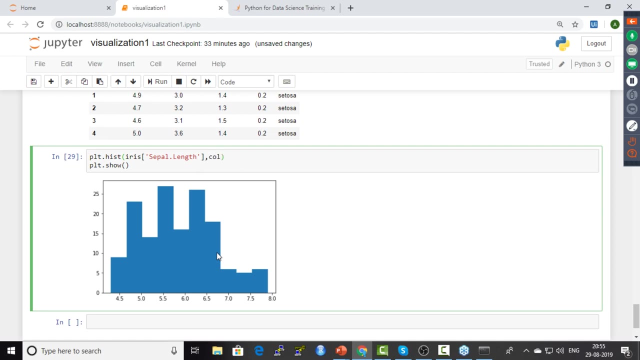 and there are very, very few flowers whose sepal length would be greater than 6.5 right, and those flowers whose sepal length is 8, those are almost non-existent right now. let's actually also go ahead and change the color of the histogram, so i'll type in color over here and i'll assign the color to be red right. so we have successfully. 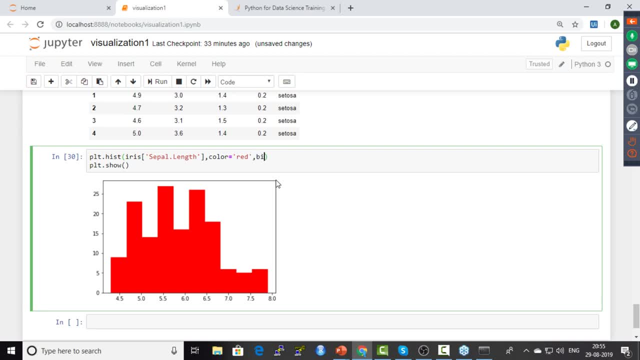 changed the color. now we can also change the number of bins over here to, you know, increase the distribution. so i'll set the number of bins to be equal to 30. right, so we can also vary the number of bins. now let me change the number of bins to be 100 and let's see what do we get. so i'll type in: 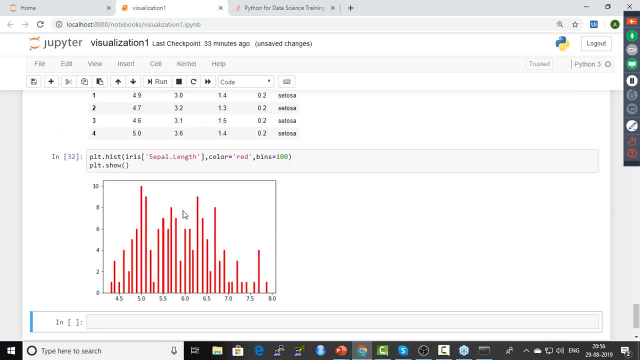 100 over here. right, so this gives us a greater distribution in the histogram right now. let me actually keep this to be 50, because 50 seems to be the perfect distribution for us right now. yep, so this is basically how we can create histograms in python or with matplotlib. now, 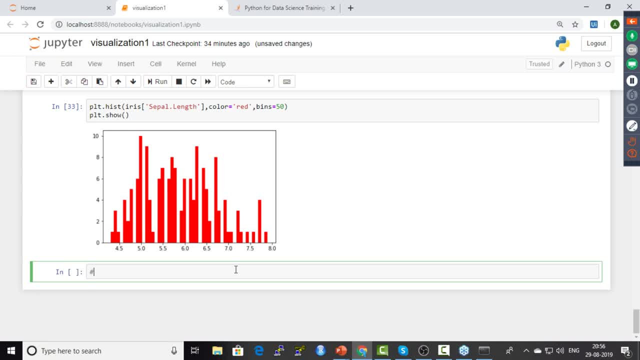 going ahead. we'll see how can we create a box plot. so i'll just type in box plot over here. now let's go ahead and, uh, create data for this box plot. so i'll create three lists. so i'll type in one, two, three, four, five, six, seven, eight and nine. so this is our first list. after that i'll go ahead. 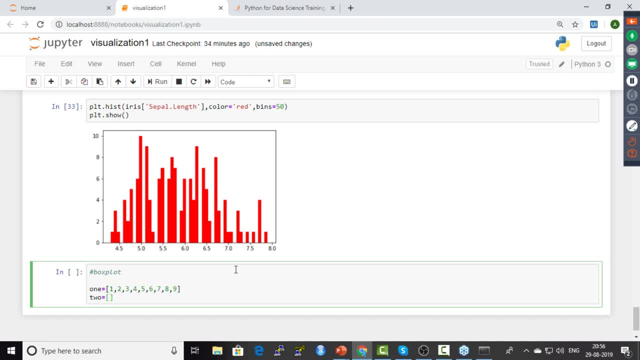 and create the second list. so in this the values would range between one and five. so one, two, three, four, five, four, three, two, one, seven. let me just count five, six, seven, eight, nine, right, let me create another list over here and, uh, this would have values between six and nine. so let 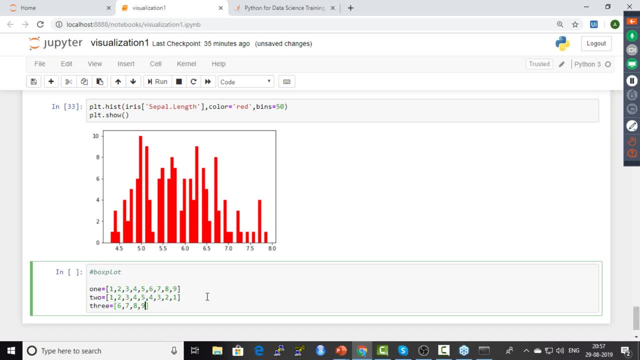 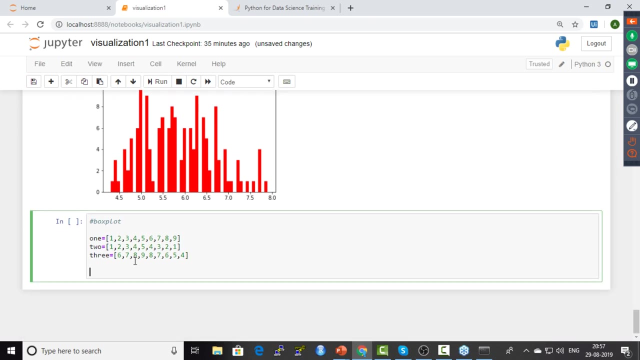 me type in six, seven, eight, nine, and there will be eight, seven, six, five. so i've got one, two, three, four, five, six, seven, eight, nine values over here, right? so i've got my data ready. now i will create a list of lists over here, so data equals list, and i'll just pass in one, two and three inside this. 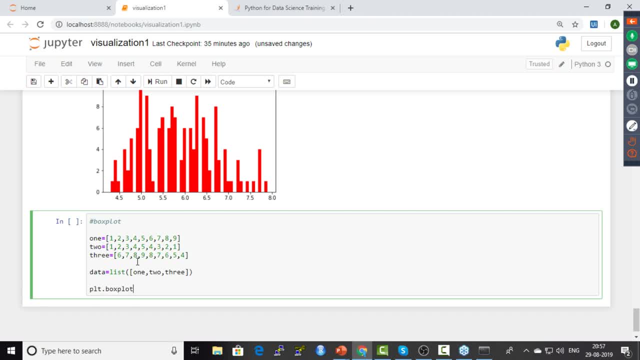 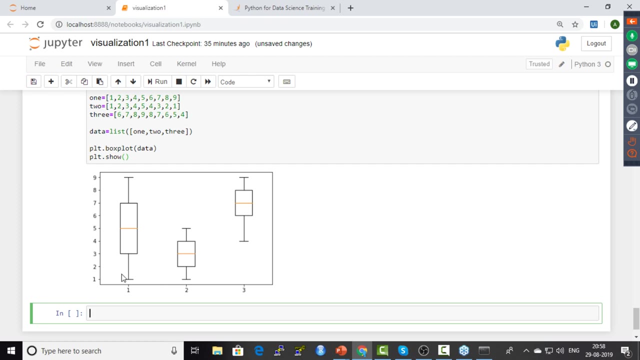 now i'll use plt dot box plot. i'll use this method and i'll just pass in data inside this again to show the box plot. i'll put in plt dot show. right, so we have successfully created our box plot over here. so this basically states that: 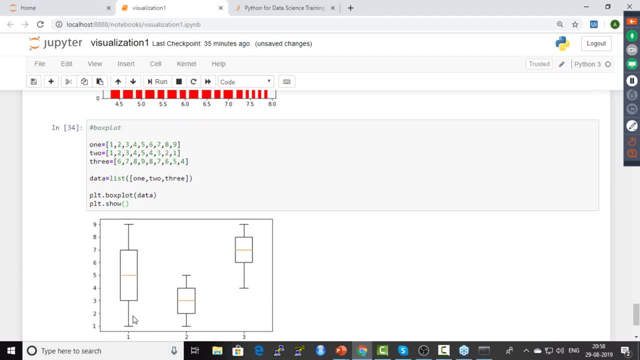 there is a greater distribution for this data. one right. so the values of, uh, this data, it basically ranges from one to nine and the median value is five. so this line which you see at the center of the box, this basically denotes the median value, and the median value for this data is five. then 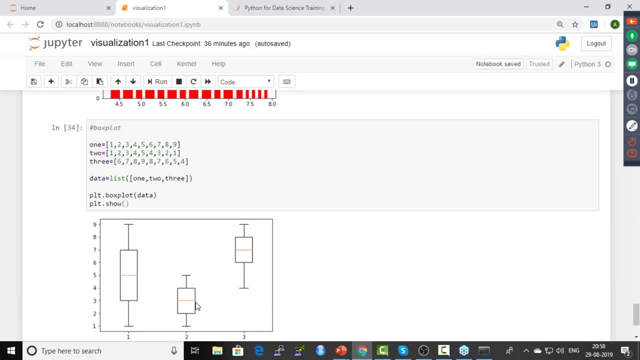 we have this box plot and this tells us that the data, it ranges from one and it goes till five and the median value is three. and then we have this over here, the data points: it starts at four and it goes till nine and the median value for this. 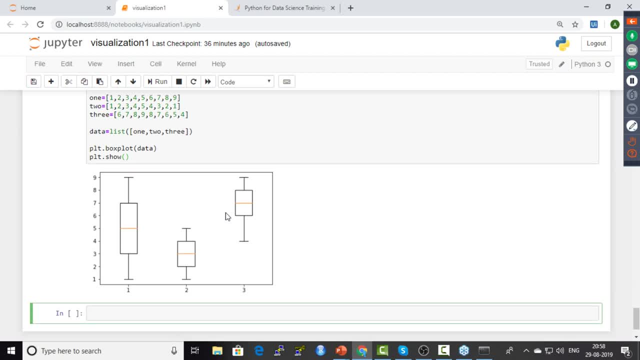 is seven. all right now, similar to box plot, we also have a violin plot. so the only difference between a box plot and a violin plot is that the shape is different. so a box plot looks like a box and a violin plot looks like a violin. so that's pretty much the only difference when it comes to the 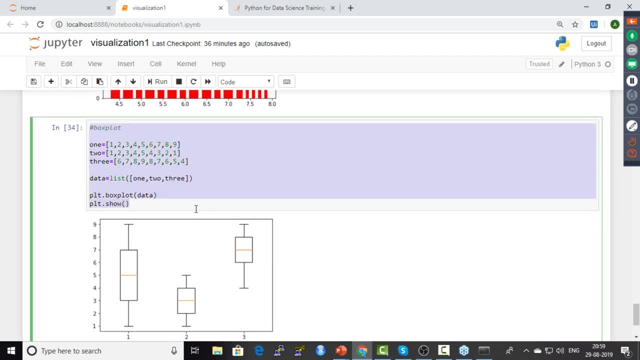 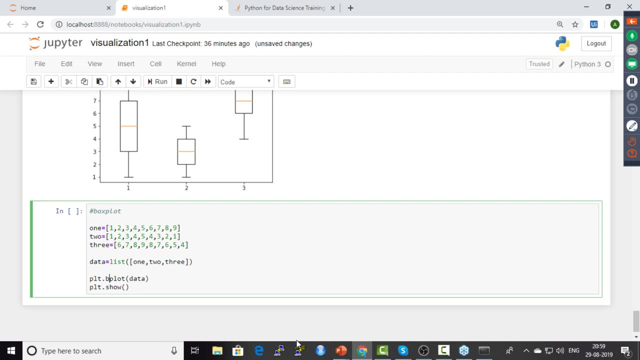 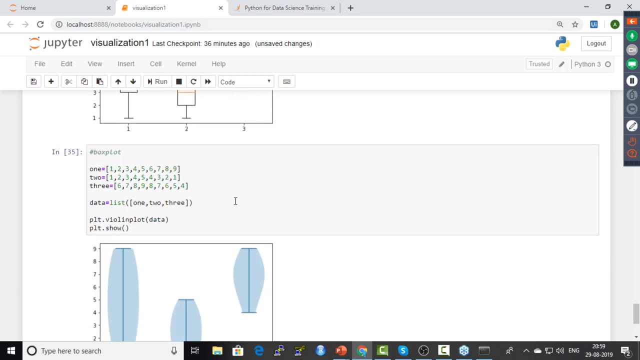 box plot in the violin plot. so i'll copy this and i will paste it over here. now. the only change which i'd have to make over here is, instead of pltboxplot i'd have to put in plt, violin plot. all right, so this is what we have over here, right? so this is the same thing, it's just that. 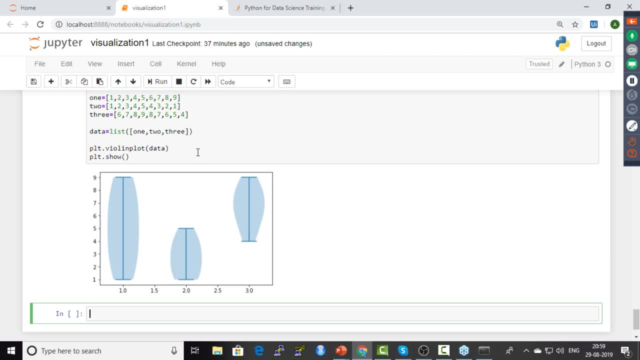 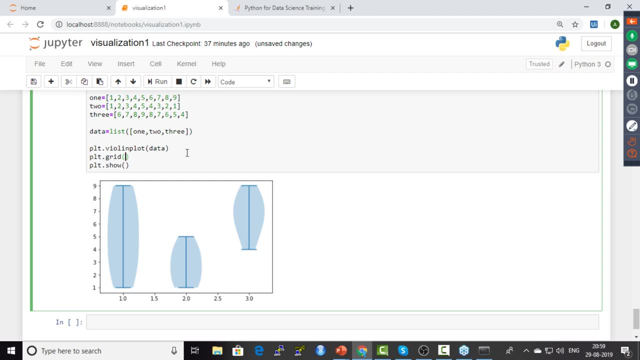 these three figures. they are in the form of a violin instead of a box. now we can also add grid to our data. so to add a grid, i'd have to use plt, dot, grid and then set the value to be equal to true. so this is how we can add a grid to our plot. now, again, let's also um add a title to this. 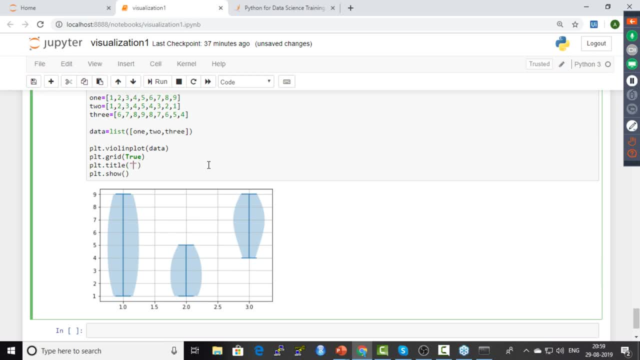 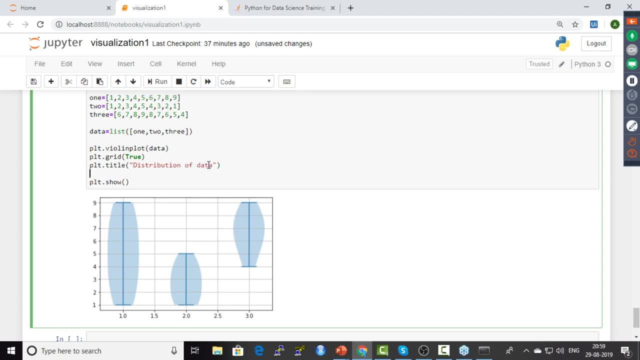 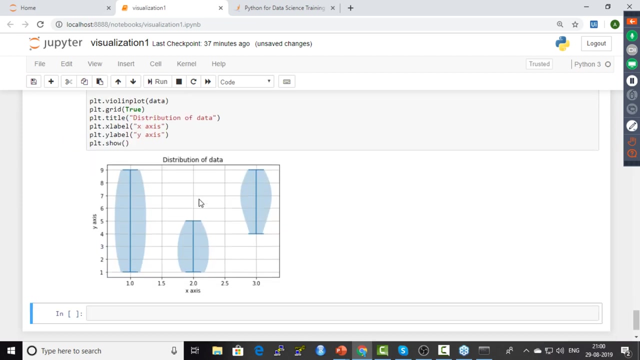 so i'll just put in plttitle and let me put in the title to be distribution of data. let me put in the x label, so pltexe label, and let me just put in this as x-axis, given the Y label over here. so PLT dot Y label and this would be y-axis, right? so 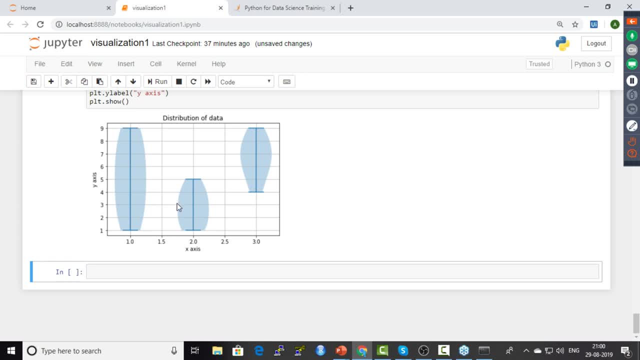 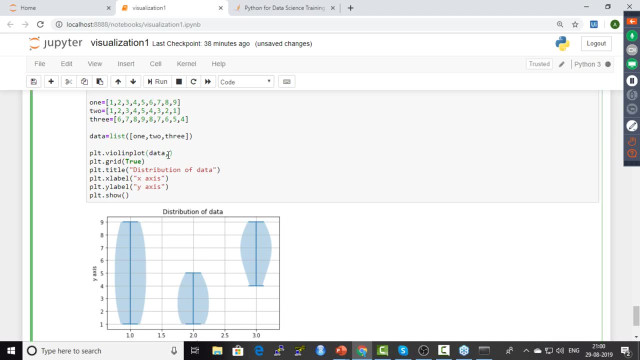 we have successfully added the title, the x-axis label and the y-axis label, now similar to box plot. we can also add a median to this violin plot. so to do that, we have this argument called as show median, and I would have to set this to be true over here, right? so we have added these lines for the median values, so not. 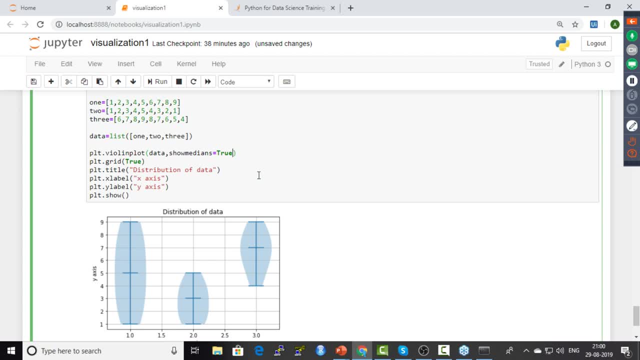 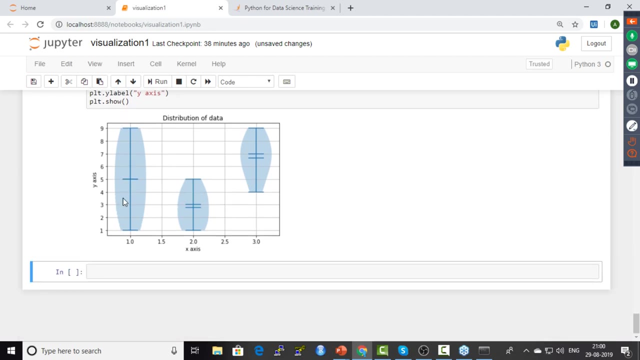 just medians, we can also show the mean value over here. so to show the mean value, we have this argument: show means, and again I'll set this to be equal to true. all right, so we've added the mean line as well as the median line. now, if 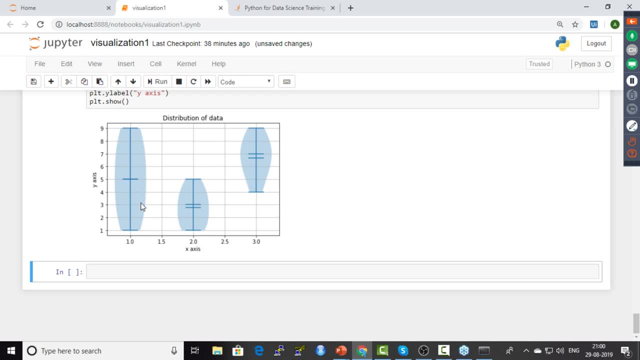 you look at this violin plot, it's a very interesting observation. so you see that the value of mean and median, you see that the value of mean and median is equal to the median value and the same for this distribution over here, right? so the mean value is Phi as well. 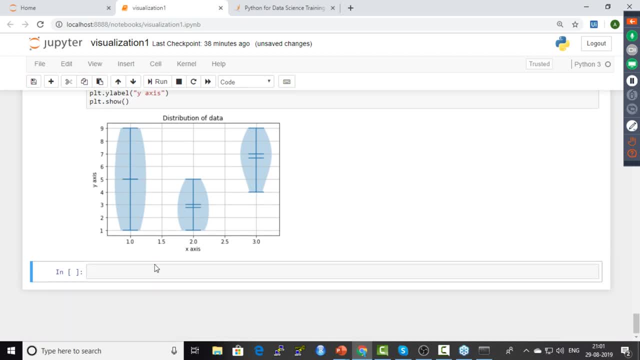 as the median value is Phi for this data, right? so we are done with violin plot as well. now let's go ahead and create a pie chart. so let me just type in pie chart over here. all right now, let me go ahead and create some data for this pie chart. 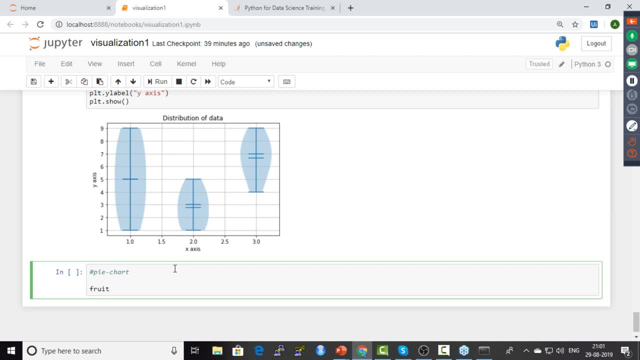 so again, what I'll do is I'll create a list with the name fruits and I'll add some fruits over here. so let's say, I'll add apple, after that I'll add mango, and then I like oranges a lot, so I'll also type in orange. and well, I've not eaten grapes for a long time, so 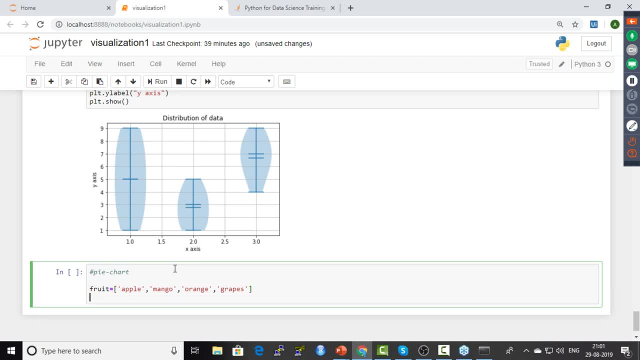 I'll also add grapes in my shopping basket, right? so we've got the first list. now we'll also add the quantity for this. so I'll type in quantity and let me give in the values for this. so let's say, I would want three thirty apples, and since I like mangoes a lot, I'd want 45 mangoes. I don't like. 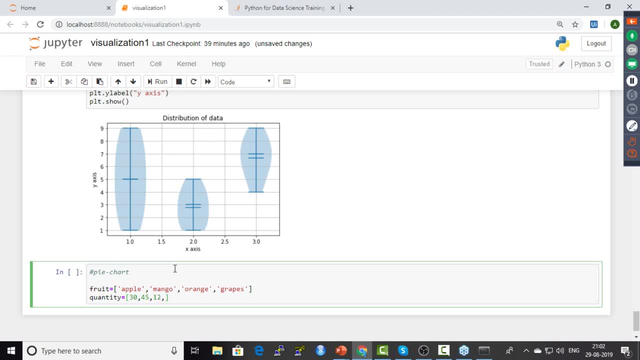 oranges, so I'll put in at to be twelve. and well, someone told me that grapes would make my health better, so I would want around 100 grapes. all right, I've assigned the values for this. now all I have to do is create a pie chart. so for 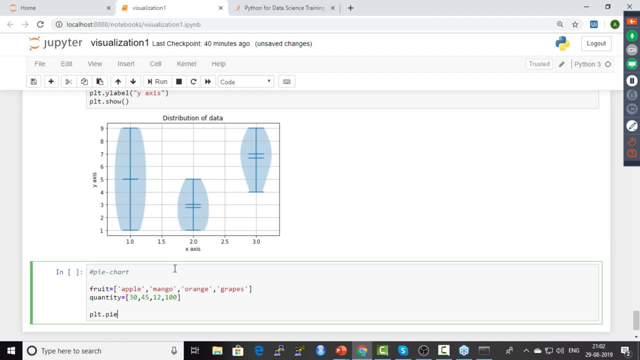 this. I'll type in PLD dot Phi and let me give him the values. so this first takes in the values. so i'll type in quantity over here and then i'll give in the labels. the labels are stored in fruit right now. i'll just type in plt dot show over here and, uh, let me create this pie chart right now. 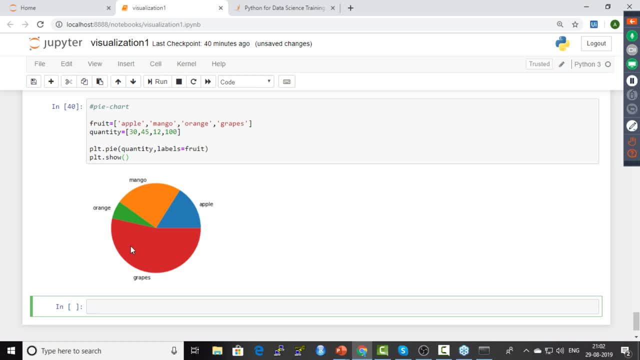 isn't this a beautiful pie chart over here, right? so this pie chart easily tells us that the major quantity of the fruits is grapes and the least quantity of the fruits is orange. now we can also add percentage over here. so to add percentage, we've got this argument auto pct and over here. 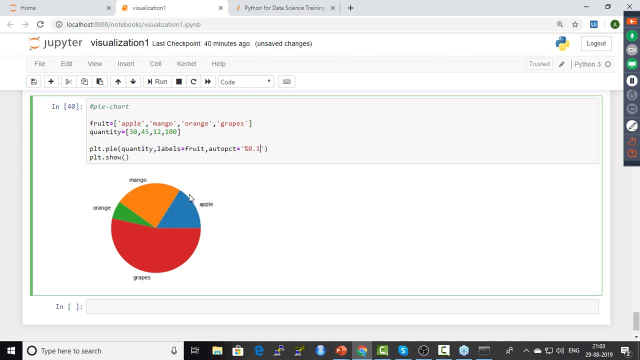 i'll just type in percent: 0.1, f, f, f, percent, percent. now let me run this. so we have successfully added percentage to this pie chart. so we see that from the entire basket, 53.5 of the fruits are grapes and the least is 6.4 percent, right, so the least amount of fruits available in the 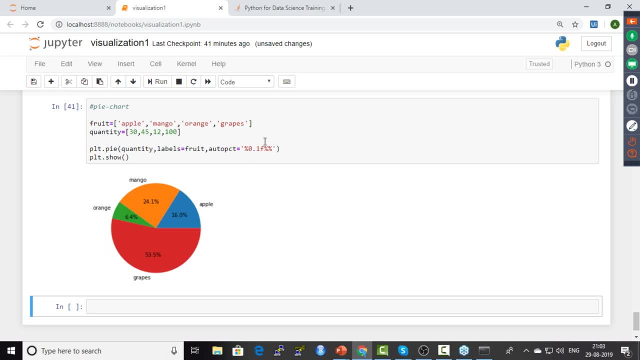 basket are oranges. now we can also add a shadow to this pie chart. so to add a shadow, i have this argument known as shadow, and i just have to set it to be equal to true right. and so let's say, if i want to highlight one of these slices, right, we can also do that. so to highlight a slice i have, 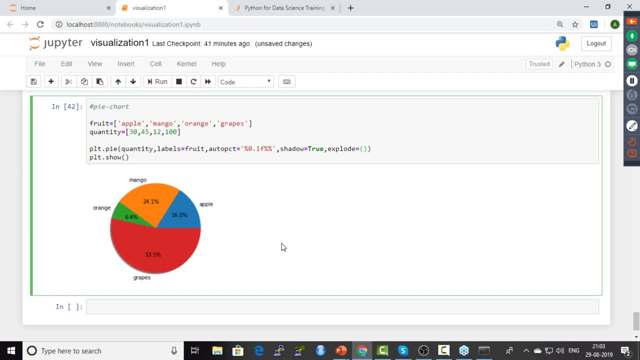 this argument called as explode. now let's say i want to highlight this slice of grapes because this is the largest piece, so what i'll do is i will type in 0 comma 0 comma 0, and then i'll give in 0.1 over here and let's see what do we get right? 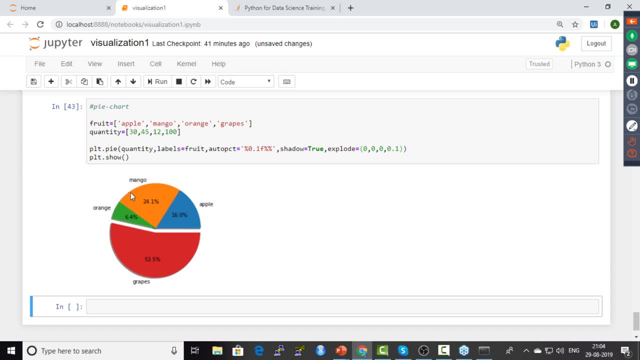 so you see that this portion over here is separated from this entire pie. now, the 000 basically means that all of these three slices would be intact together, and when i give in 0.1, this means that this original pie. now let's see if i just put it to be 1 instead of 0.1, right, so this increases. 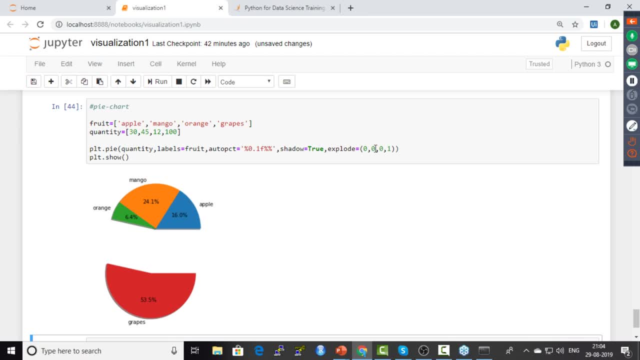 the distance between this right. so, um, now let's see if i also want to separate this over here, which basically represents mango. so i'll put in 0.1 over here and i can also separate that right. so i've also separated mango from this original pipe right now. um, a similar plot, which is, uh, you, 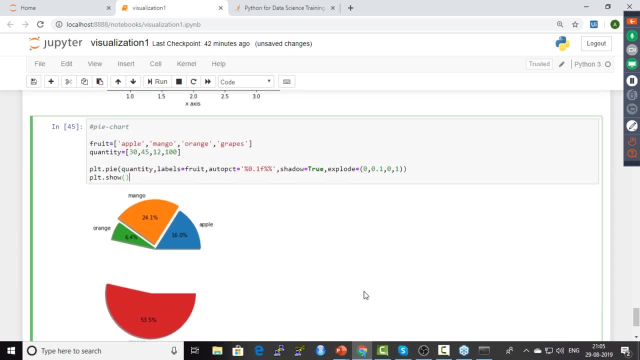 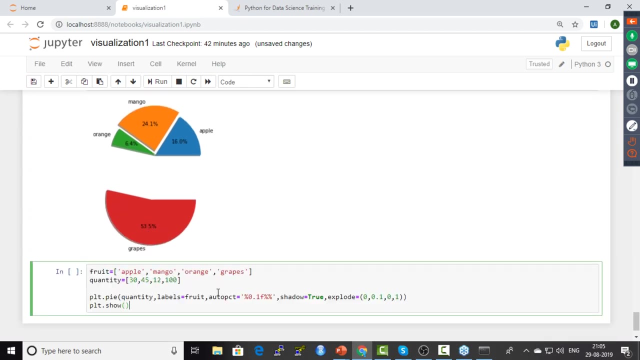 plot was similar to pie chart, as known as a donut plot. So everything is same between a donut plot and a pie chart, It's just that the donut plot looks like a donut and the pie chart looks like a pie right. So what I'll do is I'll copy all of this and I'll paste it over here. Now let me. 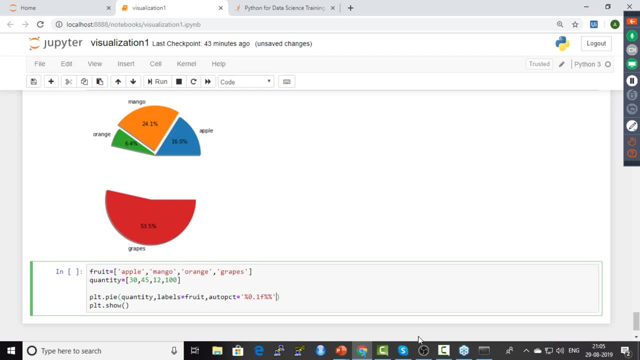 remove all of this over here. I'll remove the shadow right. So, over here, what I'll do is I'll create two plots. So this is my first plot and I will store this in pie one. Now I will go ahead and create my second plot. I'll name this second pie chart to be equal to pie two And over here. 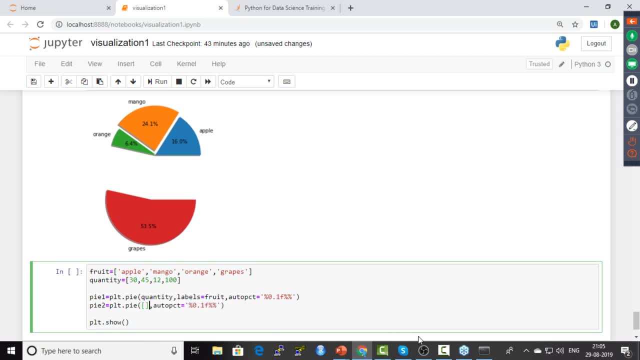 I'll just give in quantity. So let's say the quantity is equal to five over here and I will give in the color over here, right? So? um, let me also given the color. Now the color has to be equal to white, right? So now let me just 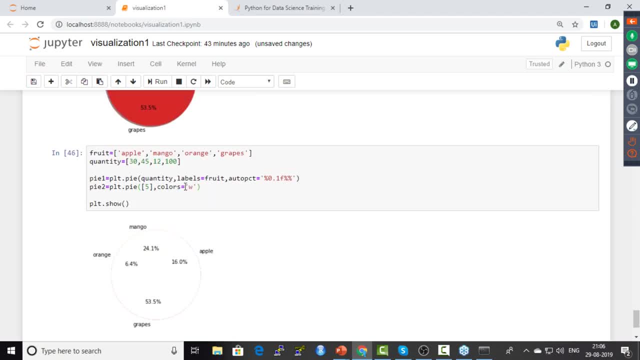 click on run and let's see what do we get over here, right? So we have this. let me remove this over here. We've got pie one, they've got pie two. Now what we have to do is we just have a white. 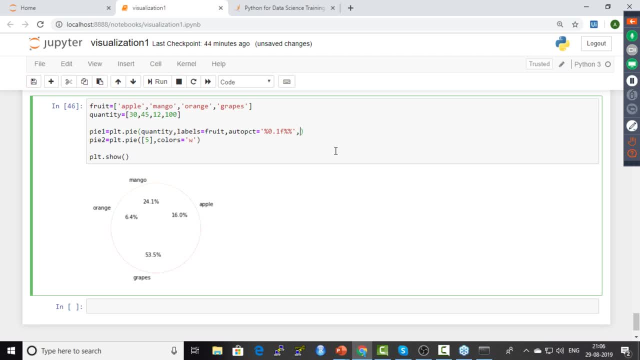 circle and we've got this over here Now we'd have to. we'll give in the value for the radius. So I'll set the radius for the original pie chart to be equal to two and I'll set in the radius for the second pie chart to be equal to one right. So 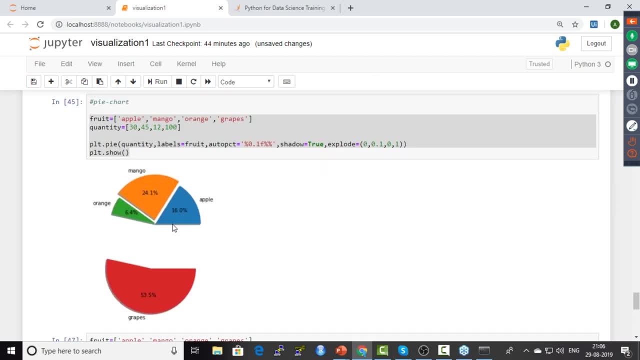 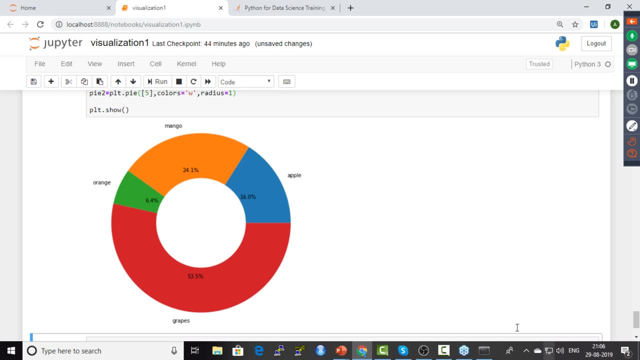 now we've got a donut plot and it looks like this, right? So if you have a glance at this and this, it's pretty much the same. The only difference is this looks like a pie and this looks like a donut. Now, all we did is we created two pie charts over here. The first pie chart is the. 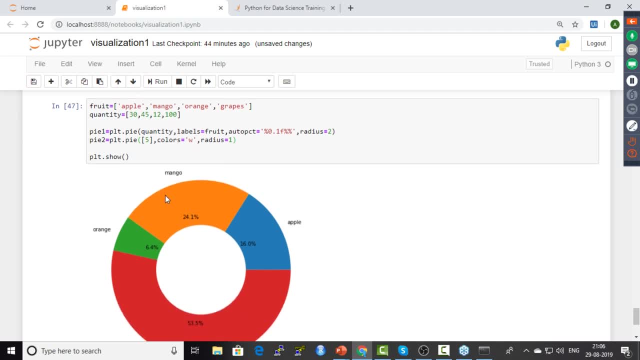 original one. The second pie chart is the original one. The second pie chart is the original one. The third pie chart is just a white circle over here, right? So this is a white circle. We've assigned the color to be equal to W and the radius of this inner pie chart should be lesser than the. 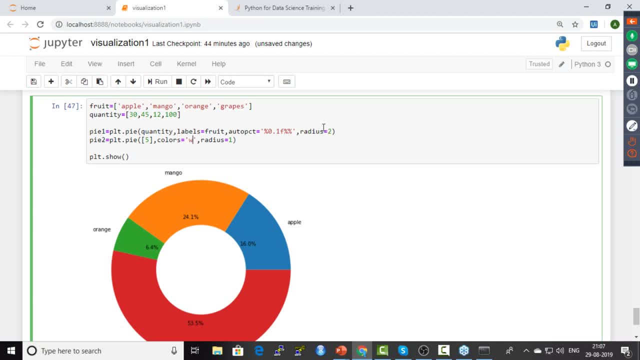 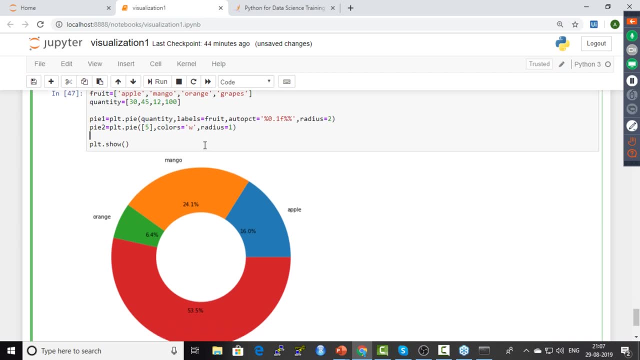 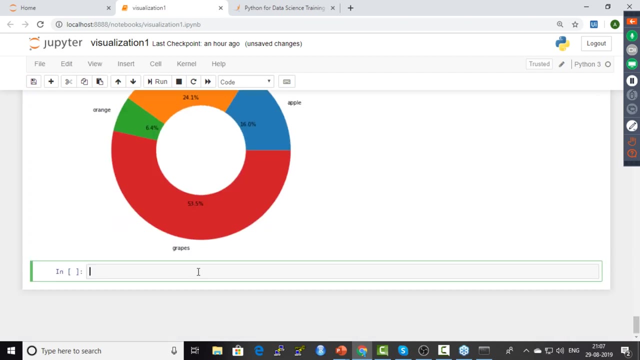 radius of the outer pie chart. So, for the outer pie chart, I've assigned the radius to be equal to two, and for the inner pie chart, I've assigned the radius to be equal to one, Right now. Yep, So this is how we can create a donut plot, And then, finally, we have 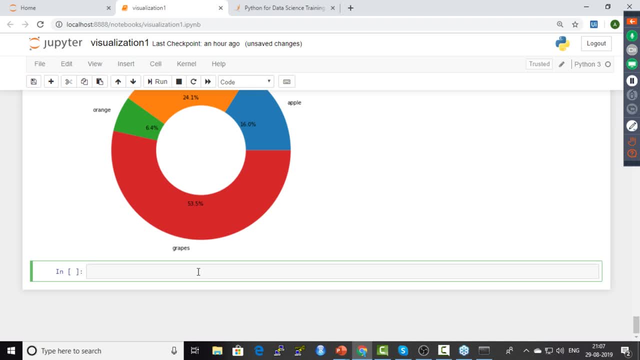 um, something known as an area plot. So let's go ahead and also create an area plot over here. So, um, let me create some values. Let me just type in area plot and create a bunch of values over here. So let's say, X axis, it goes from 10 to 90. So I'll type in 10,, 20,, 30,, 40,, 50,, 60,, 70,. 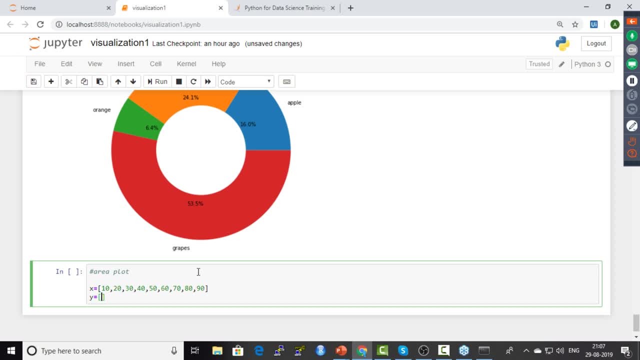 after that I'll give in values for the Y axis. So this would be, let's say, one comma, 1, 2, 5, 6,, 4,, 7, let's see how many values again: four, five, 6,, seven, including charges, And then I'll 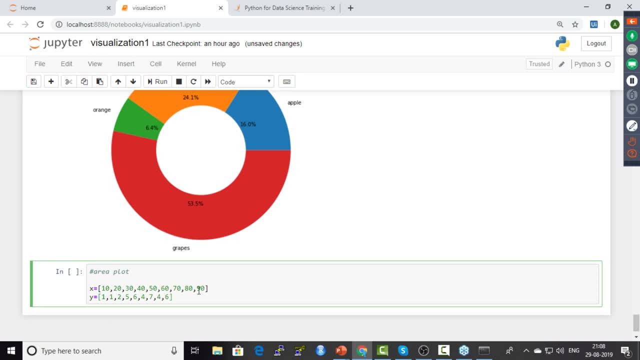 given a, I'll given a x, six, 10, 20,, 30, x. four, five, 6, 7,, 8,, 9, 8 etail. have those weights. Let me go ahead Then create this area plot. Right now I'll just type in p, l, g, dot stack plot. so my sorry plot right by net worths, which is actually a full. I'm not saying you should just say I'll say go for All right, Now let me go ahead Then create this area, a plot. Okay, All right. 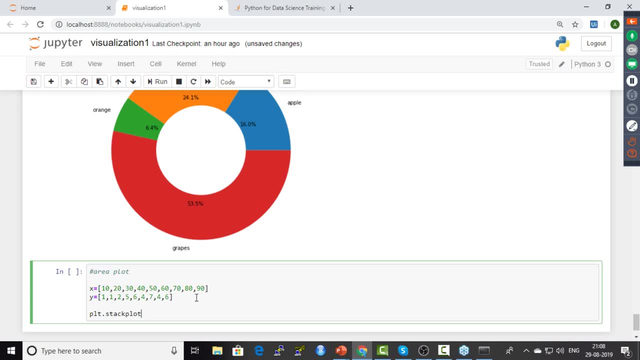 So I'll just type in P l t, dot. stack plot, area plot, dot. light up. propia plot is put on here and my dot stack plot. so to create an area plot. we've got this method known as stack plot, and i'll give in the values for x and y. after that i'll just type in: plt, dot show. right, so we have. 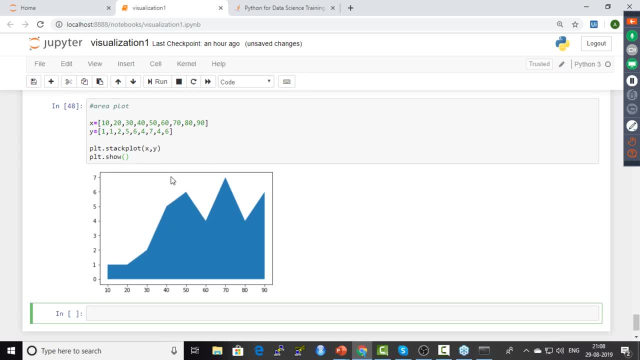 successfully created this area plot over here and this looks something like this. so this area plot is very similar to histogram, right? so the area plot and the histogram, both of them show the distribution of your numerical data. so if we look at this, we basically understand that, you know, there is a greater distribution or there is a greater frequency of the higher. 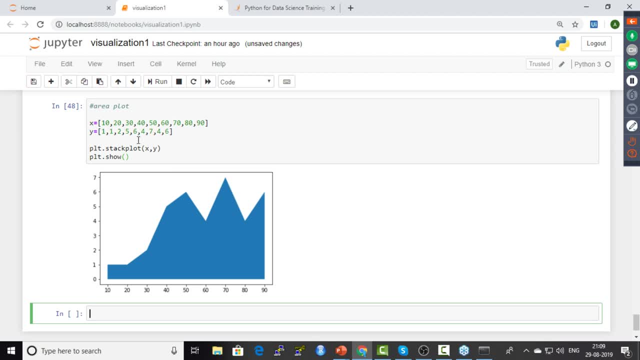 order numbers. right, if we look at this as well, so we can get to know that, right, there are two sixes, there are there is one seven and there are two fours over here. right, so this is what this tells us. right, there is a greater distribution of the numbers after. 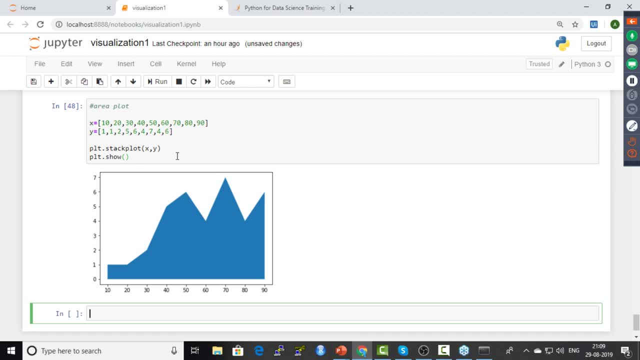 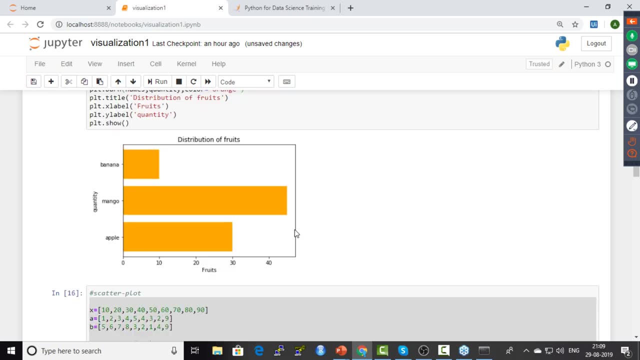 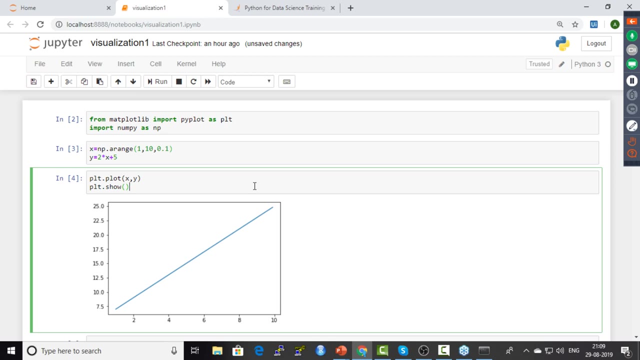 five, right, so this is basically how we can create an area plot, right? so, um, yes, guys, so, um, this brings us to the end of the session, and, uh, in this we've comprehensively understood about a lot of geometries. so we started off with the line plot and then we learned how to customize. 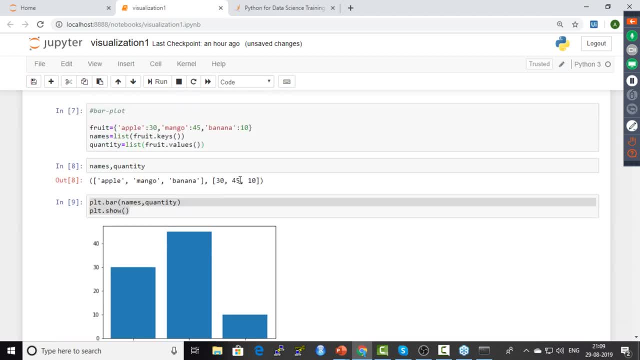 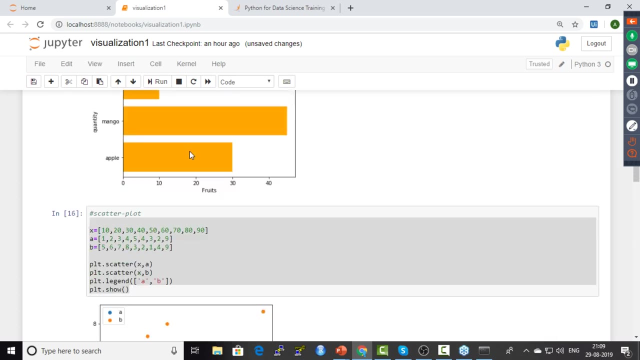 the line plot. after that we uh worked with the bar plot. now you guys have to understand the difference between a bar plot and a histogram. so a bar plot is used for categorical values and a histogram is used for numerical values. so this is the basic difference between a bar plot and a scatter plot. so after that we also learned how to uh create a. 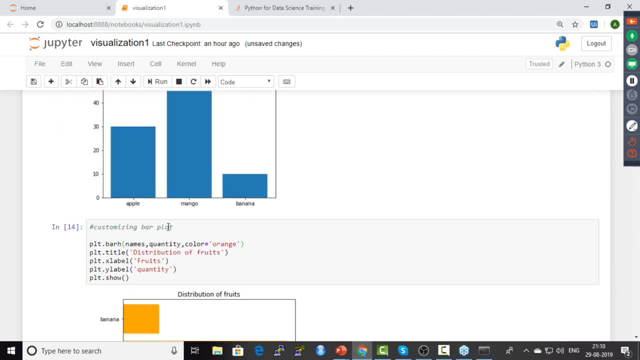 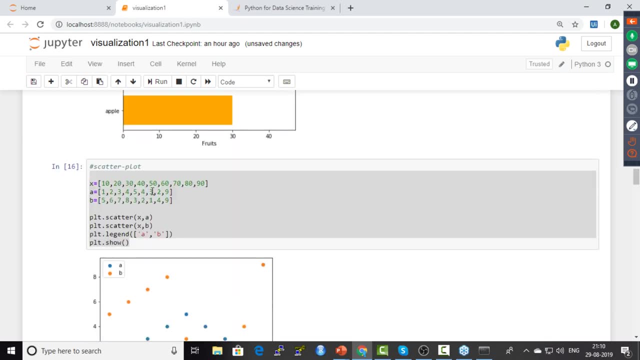 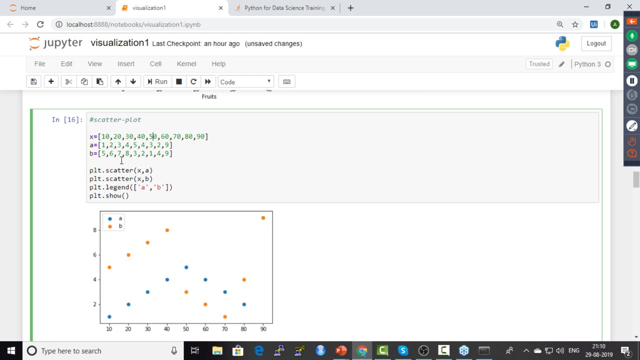 horizontal bar plot. so the only difference between a vertical bar plot and the horizontal bar plot, the syntax would be so: over here you will type in pltbar and over here you will type in pltbarh and then you will create a scatter plot. so, um, we can create a scatter plot by using this command. 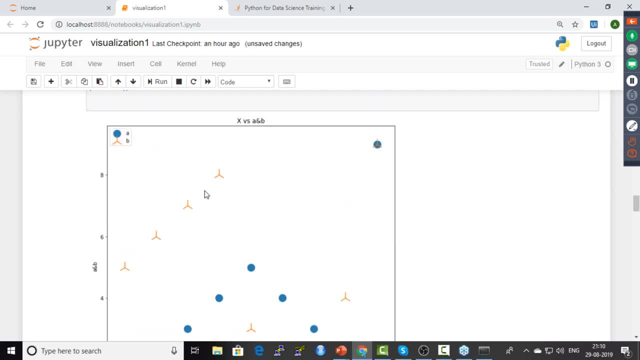 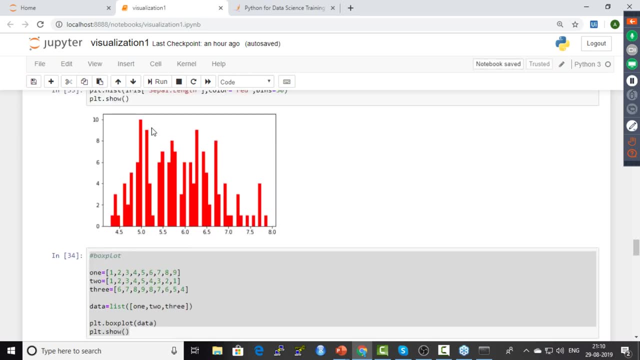 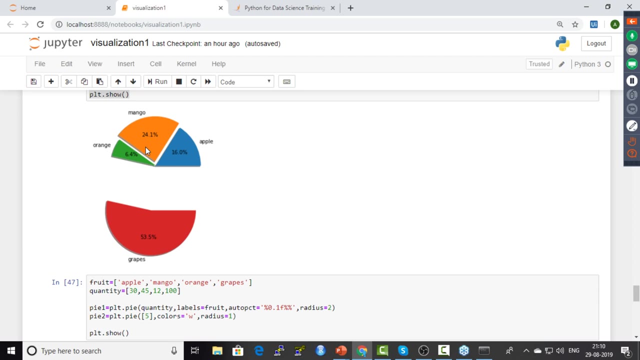 and then we saw how can we change the size and the you know marker style for these scatter plots. after that we created a histogram, and then we also created a histogram on top of a data set, and then we went ahead and created some box plots and violin plots and then we finally understood. 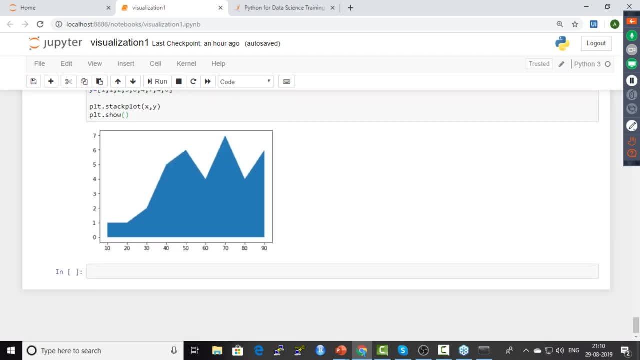 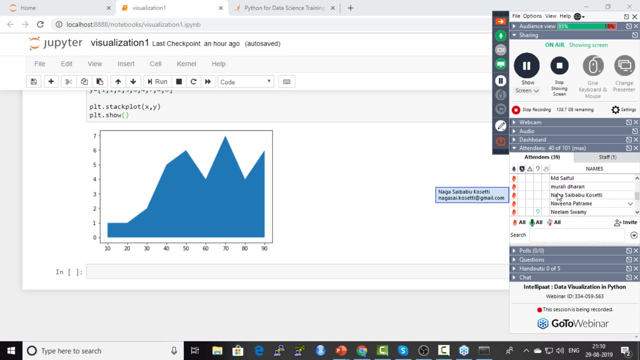 about pie charts and area plots. right so, um, guys who are attending the webinar. if you have any questions, you know you can ask me right now. right so, um, people who have questions. so let me actually unmute you guys. uh, hi, can you listen to me? yes, um, just um. yeah, i'm sorry, i'll be back in one second. 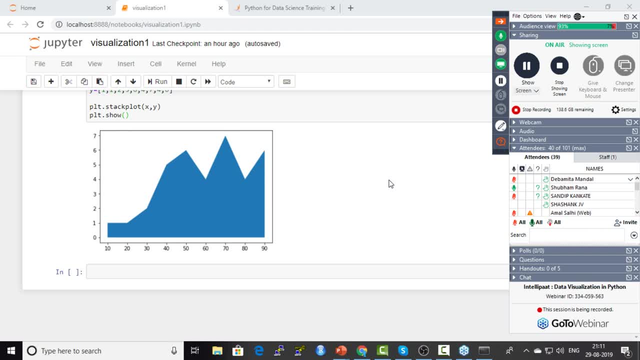 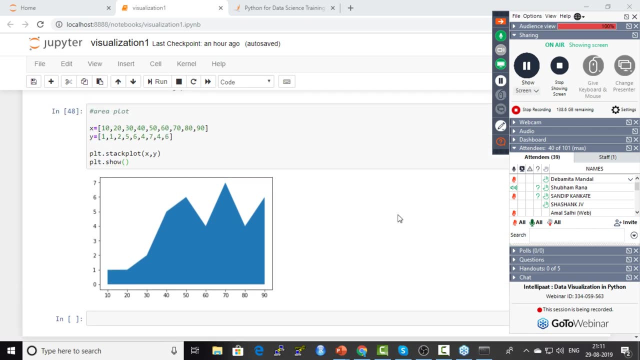 yeah, hey, um, so i believe this is Shubham Rano. uh, yeah, may i know your name? yeah, um, so i'm Bharani over here, hi, so this was a very nice session. uh, so it was quite informative. so now i wanted to know something that, uh, whatever the donut plot that you were creating over there, right? 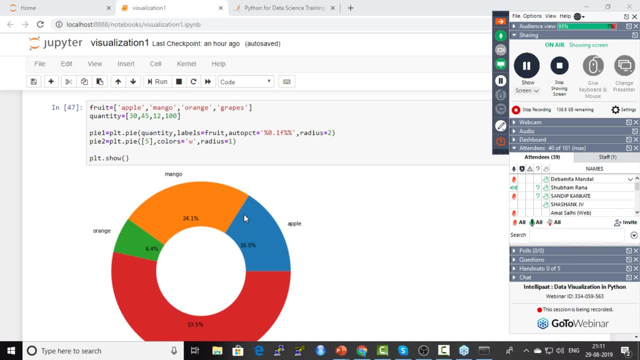 yeah, you mean. so correct, correct? uh, what if i want to add another circle in that donut, inside the donut plot? how would i do it? okay? um, So, as you see over here, to create a donut plot, I've just created two pie charts. 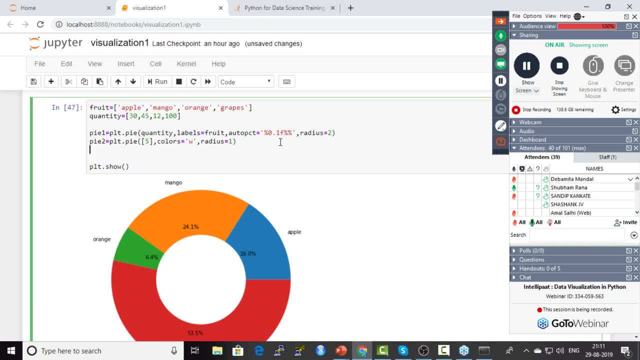 So to add another circle inside this, I'd have to add another pie chart. So what I'll do is I'll add another pie chart. I'll name this to be pie three and I'd have to do the same thing. So I'll type in pltpie over here. 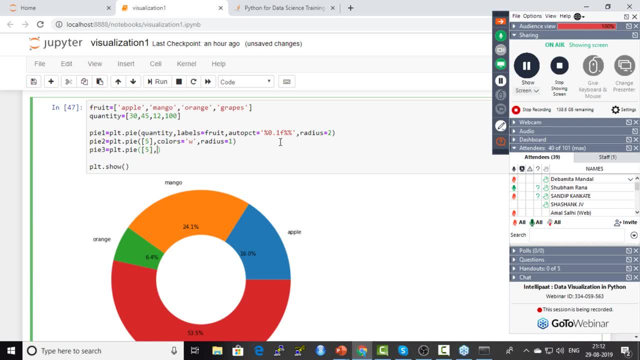 I'll give them the size of this, which will be five again, And then I'll give it a different color. So I'll use the colors argument and let me give this a blue color over here. Now, the important thing to note over here is the radius of the inner circle needs to. 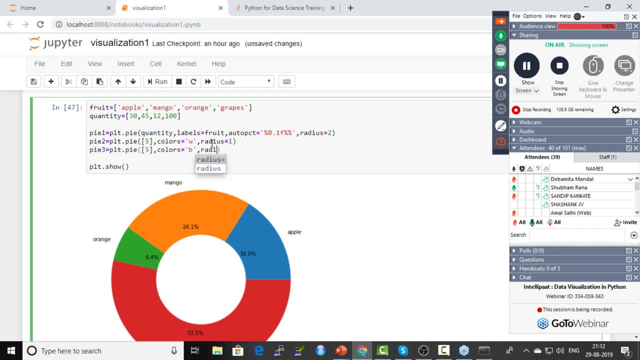 be lesser than this radius over here. So this time I would set the radius to be equal to 0.5, right? So this is our outer circle, whose radius is two, And then we have this inner circle, whose radius is one of that we have, we are creating this. 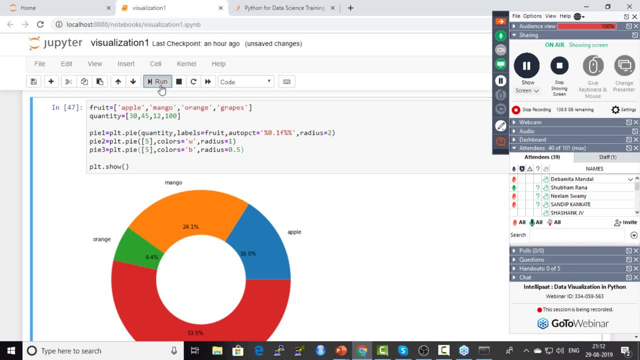 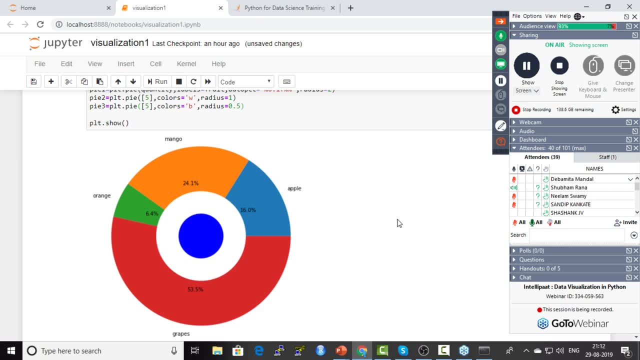 new circle inside this, whose radius is 0.5.. Now let me click on run right, So we have another circle inside this. donut plot Seems convenient, Correct. Okay, Let's do one more if you don't mind. 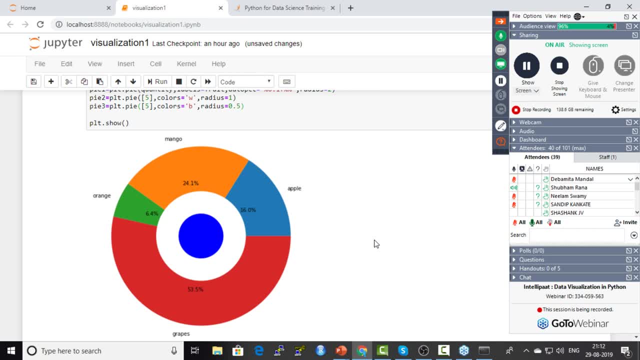 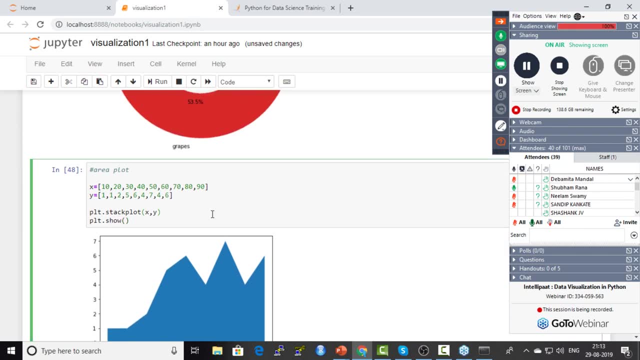 So can I add a line plot on top of the area plot? Yes, you can do that, And it's a very simple step over here. So all you have to do is below this, you'd have to type in pltplot, because this is how. 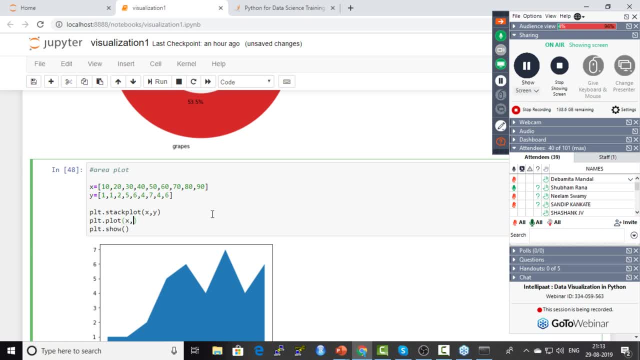 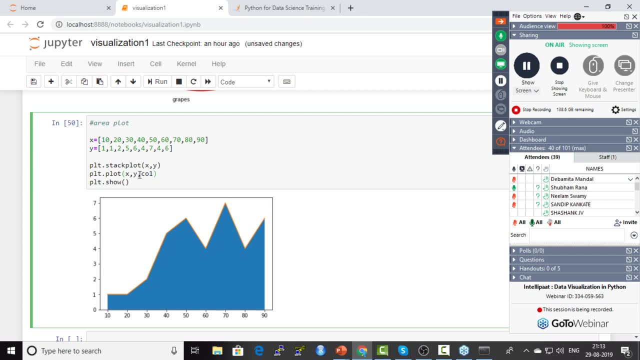 you create a line plot And then you're given the same values over here, So X, comma, Y. Now I click on run. Now you can also change the color to this line. So let's see, I'll type in color over here and I will give in a green color to this right. 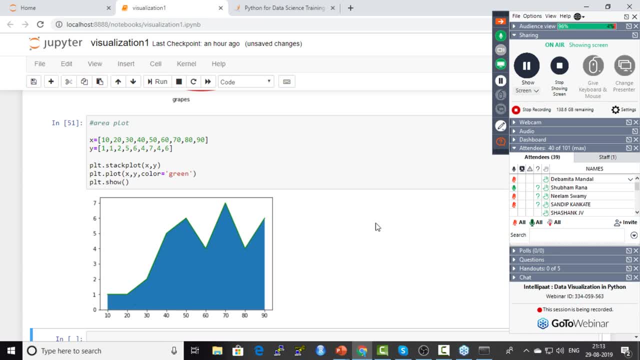 So this is how you can add a line plot on top of this area plot. So does that help you? Yeah, Yeah, It sounds convenient, Correct. And about the pie chart: how do I change the colors in it? Right, So you're talking about this pie chart over here? 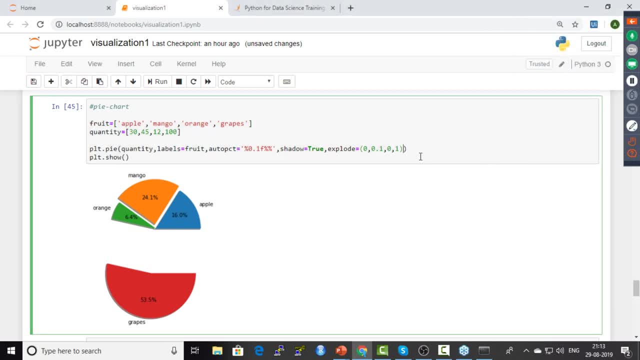 Right, Okay, So for this, what you'd have to do is you'd have to use the Okay. Okay, So you'd have to use the colors parameter, as we've been using, for you know, other geometries as well. 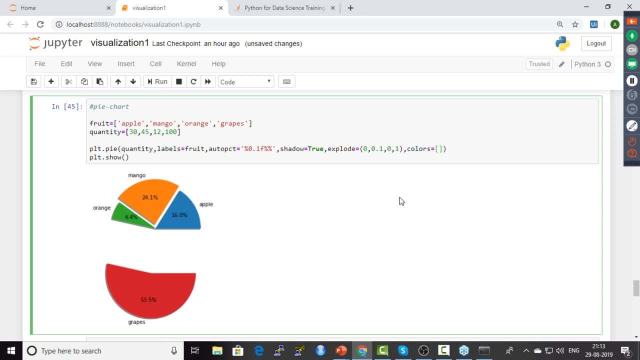 And since we've got four slices over here, what I'll do is I will give four different colors. So let's say, the first color which I given is black, The second color which I given is gray, And then I give in yellow, and then let me just give in green over here. 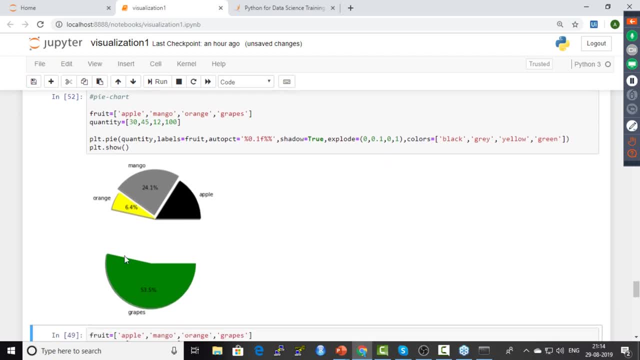 Yeah, Yep, Right, Okay. So this has changed, Right. So all you have to do is you'd have to check the number of slices you have. So if you have 10 slices, you have to create a list which comprise of 10 elements. 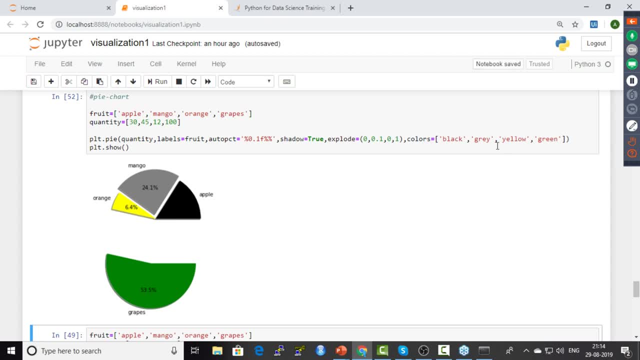 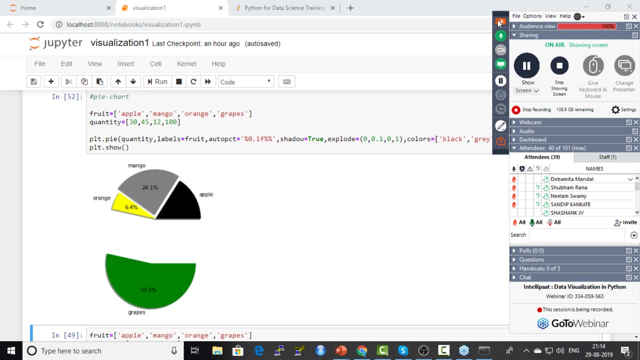 If you go out five slides, you'd have to create a list which comprise of five elements. All right, So is that it? Yeah, That's it, That's it Okay, All right, Yeah, Yeah, All right guys. 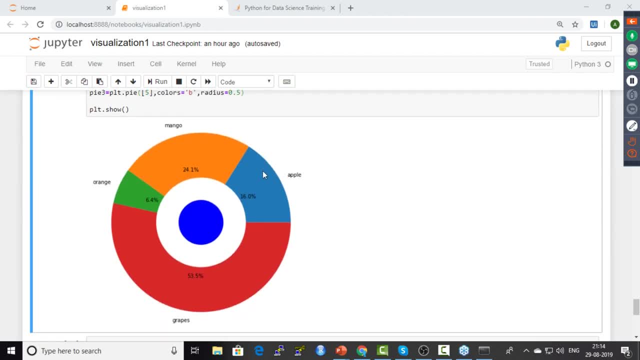 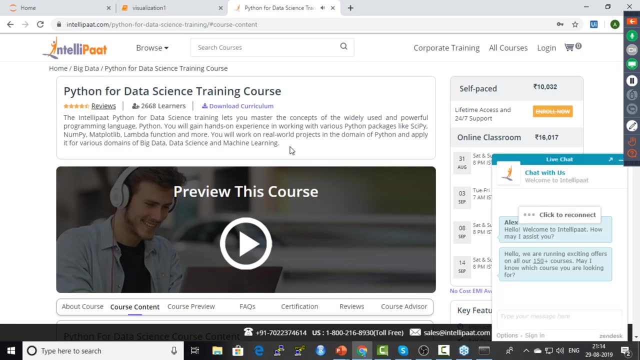 Then. So no one else has any more doubts, What I'll do is: yeah. So this brings us to the end of the session, now you know. so just for an info over here. So Intellipaat actually has this Python for data science training course. you know where? 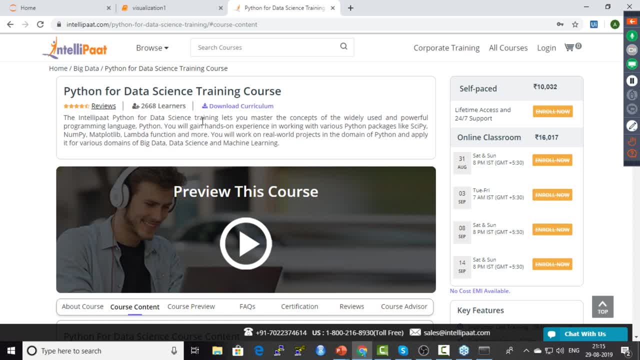 you can learn all the major concepts of Python and data science thoroughly. So Intellipaat has done a lot of research. So Intellipaat has consulted industry experts who've, you know, worked with data science. you know they've done a lot of research. 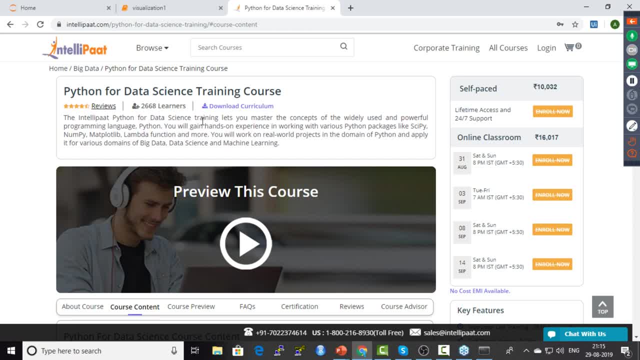 Okay, And as data scientists in top companies, and in consultation with them, they've come up with this Python for data science course which, will you know, given 360 degree proficiency in data science. All right, So let me actually go through this course content over here. 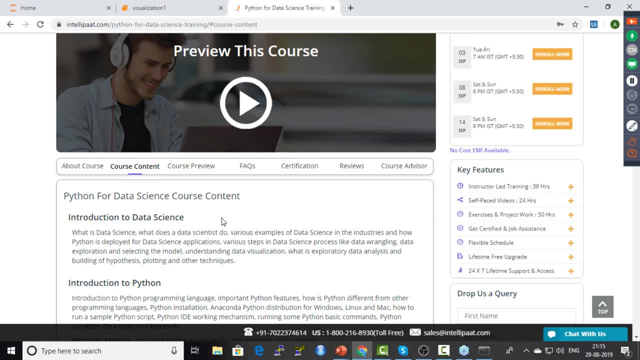 So you'll start off by understanding the basic concepts of data science. You'll understand what exactly is the need of data science. So why did data science come in? And then you look at various applications of data science. you'll understand how is data science is used in different sectors. 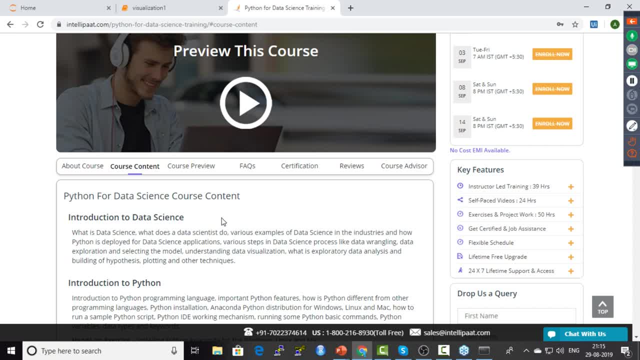 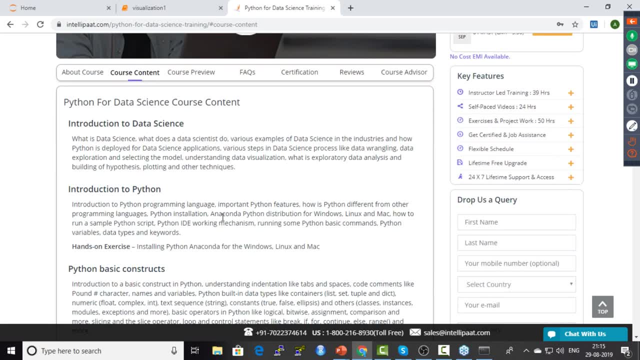 So let's say you're working in a tech industry- Okay. So let's say you're working in a telecom sector, or you're working in healthcare sector. You'll understand how is data science used in all of these different sectors. After that, you will understand the basics of Python. 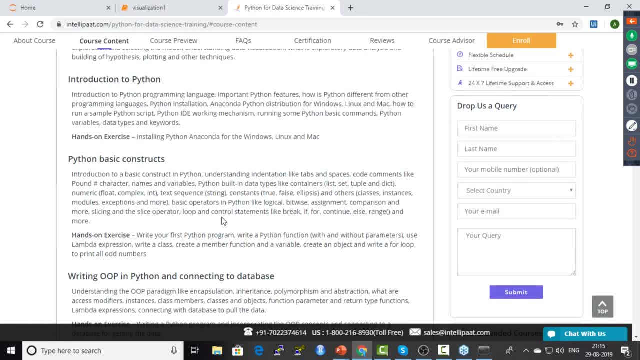 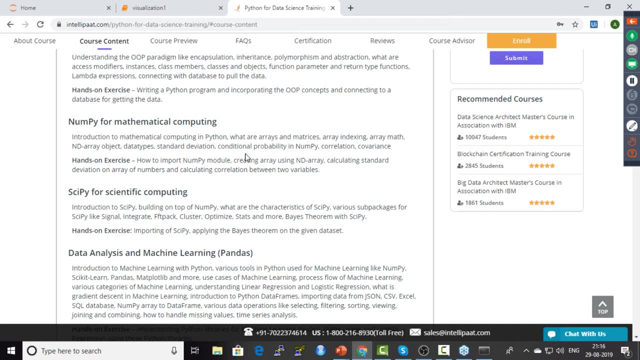 So you will understand about the different data types, how to install Python, and then you'll work with looping and control statements. And then we've just worked with the NumPy package over here, right? So you will comprehensively learn about the NumPy package and how to do mathematical computing. 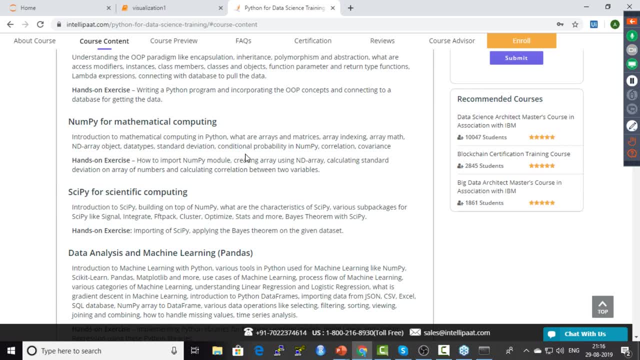 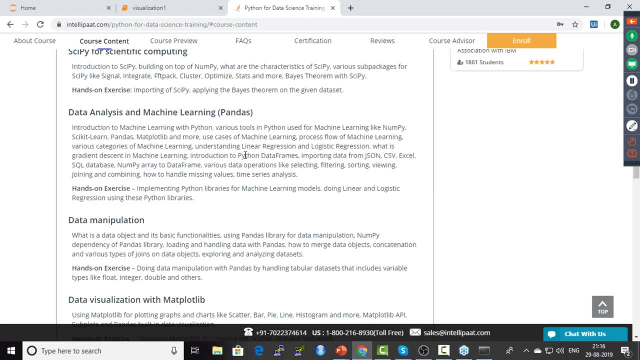 with NumPy. And then there is something called SciPy, which is built on top of NumPy. Okay, So over here you'll see how to do scientific calculations with SciPy, And then you've got the machine learning concepts over here, right? 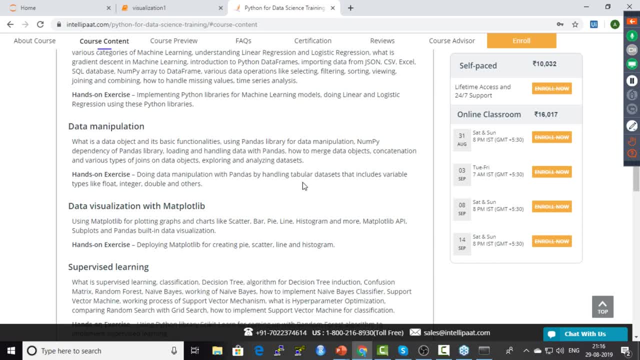 So this is where you learn how to do data wrangling and data visualization. So you'll see how to manipulate the data with the help of the Pandas library. You learn how to extract the data, You learn how to cleanse the data, You learn how to find the outliers and all of that stuff. 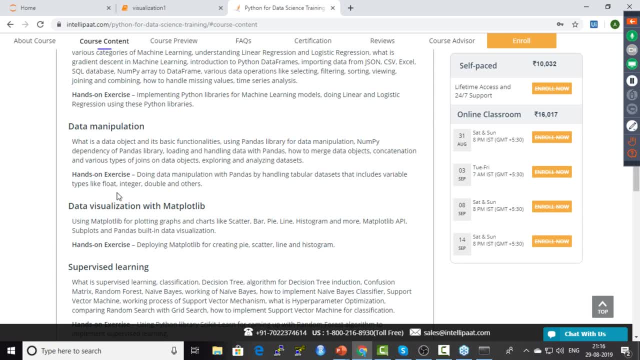 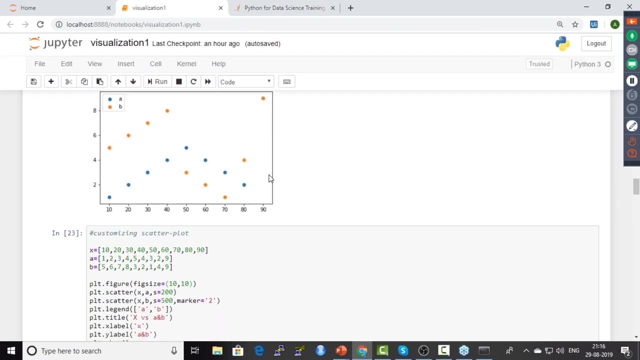 Right, And then Okay, Okay, All right, So, and then they've got the. so data science with Matplotlib. So over here, you know you so just what we've done. over here you'll comprehensively learn how to create different plots, right. 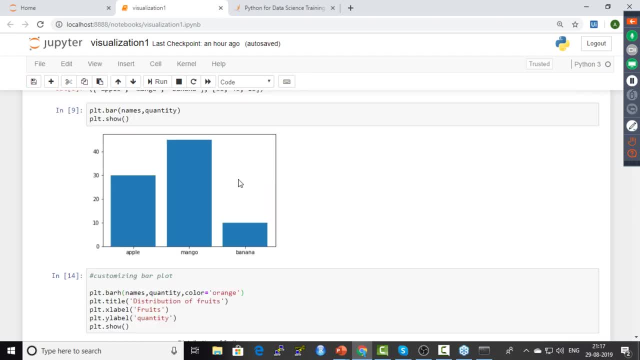 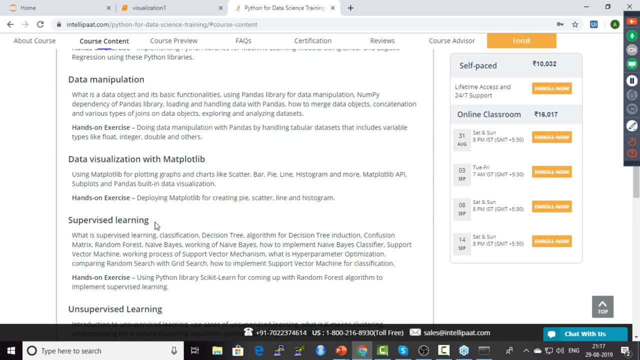 So this was just a demo over here, where you know you saw a simple example for each of these different plots. So in this course you'll comprehensively learn about different plots. right, You'll learn about different aspects of box plot, different aspects of donut plot and. 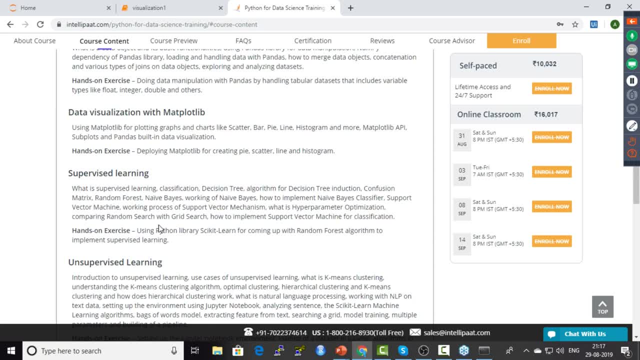 different aspects of area plot And once you're good with this stuff, you'll comprehensively learn about machine learning, So we'll start off with supervised learning. You'll understand about classification and regression and different classification algorithms, So you've got algorithms such as decision tree, random forest, Naive Bayes and SVM. 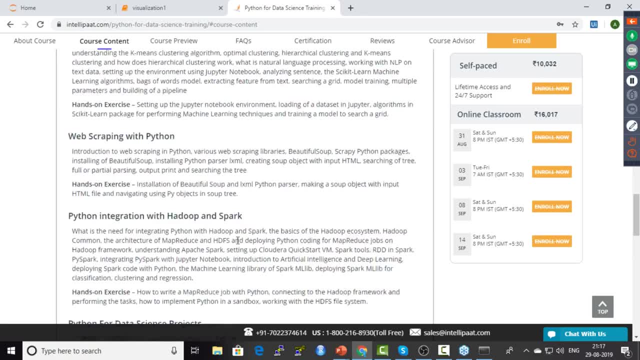 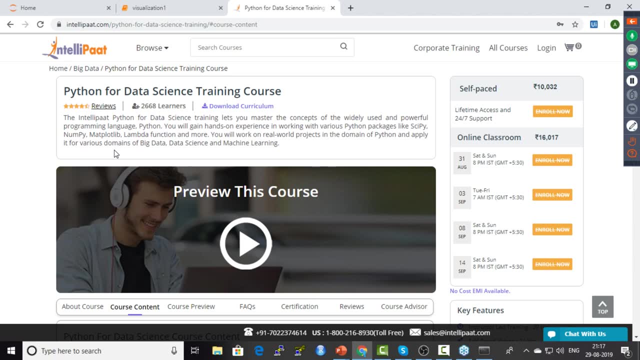 You'll comprehensively learn about this, right? So these are all of the things which you can learn with this course, right? So if you're interested in learning about data science and how to implement all of these data science concepts with Python, then you can check out the description which would 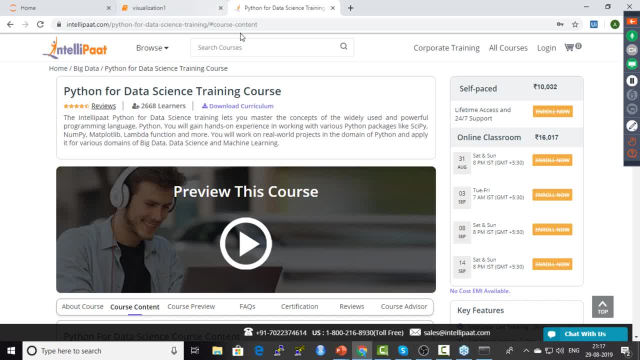 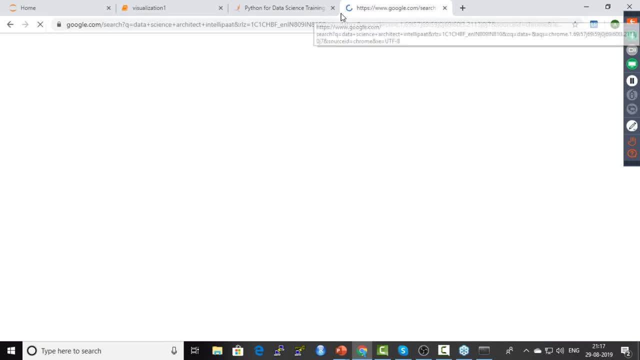 be posted in the link over there right, So also you can check this over here. Now the Intel part also provides the data science architect course, So let me just open that up and let me show you what is so what is so amazing about this? 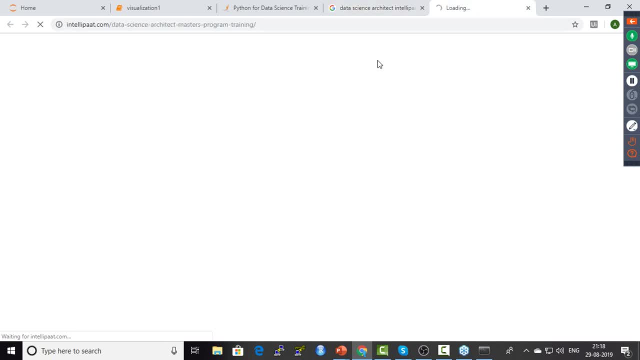 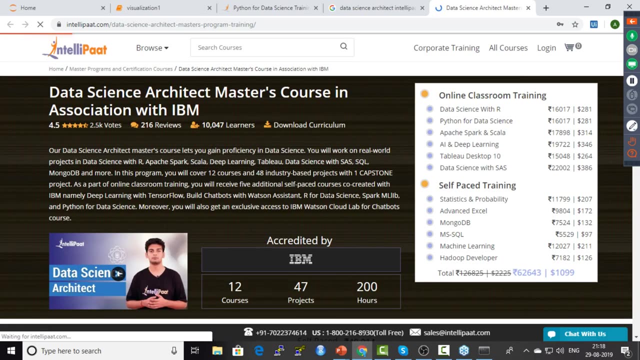 course over here, right? So the best feature about this data Science architect course by Intel path is that this is a. you know, this course has been created in consultation with IBM, in association with IBM, So you would actually be getting a certificate from IBM when you complete this course. 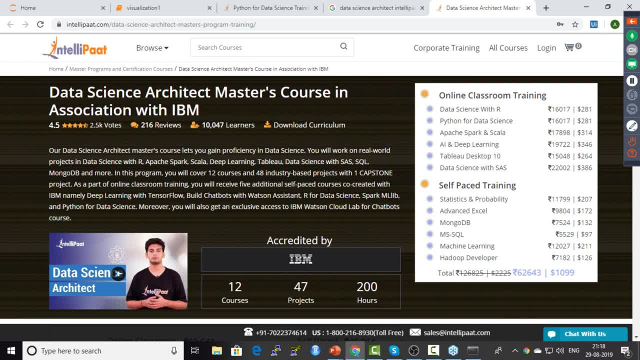 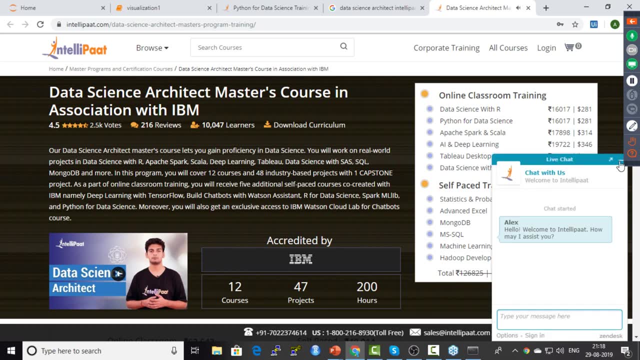 Now, that is very good, Isn't it Right? So this course basically comprise of 12 modules in total, where there are six instructor led modules and six self-paced modules. So along with this, you will also have Multiple assignments. you will have multiple projects, so that you know you have more. 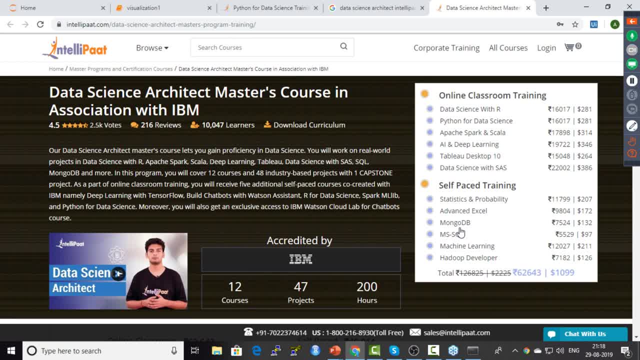 hands on expertise. So in this course you will basically start off by understanding the top three analytical tools used in the industry. So you will start off by uh. start off with the data science with our course where you learn how to do our programming and how to do how to implement data science concepts. 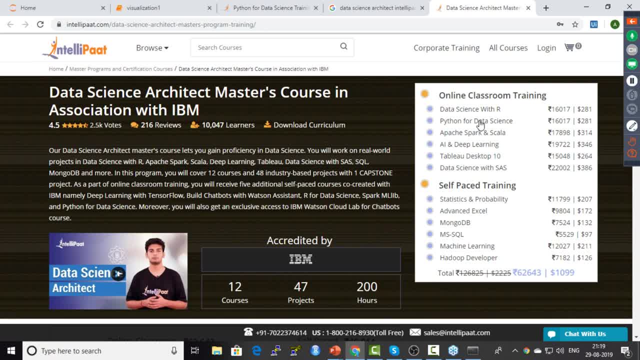 with our, and then you will uh start with the Python for data science course, but you will comprehensively learn about Python programming And also how to do statistical Analysis with Python. and then you learn data science with SAS, but you learn SAS programming. 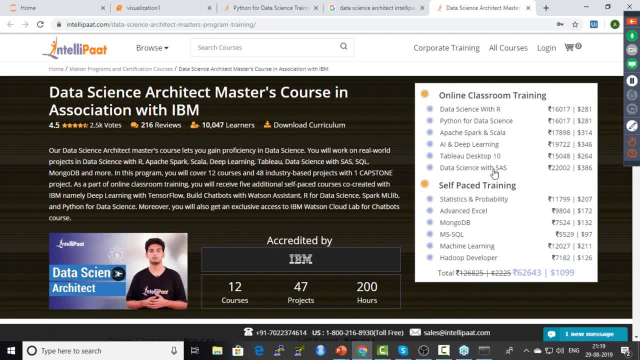 and um. you know how to do regression analysis and classification analysis with SAS. Now, once you're good with these analytical tools, you will get on with big data. So you will see how to process big data in real time with Apache, spark and Scala. 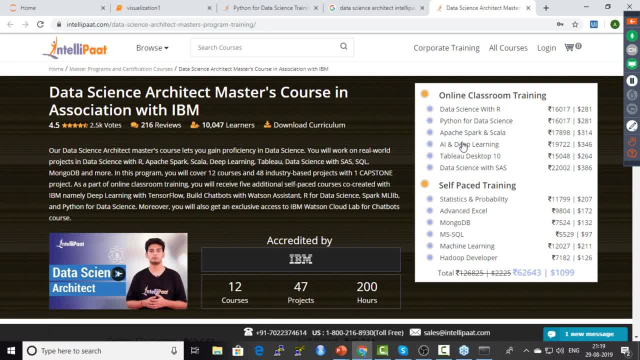 And to be a complete data scientist, you would also need to have a good grasp on the deep learning concepts. So this Uh Data science architect course also provides the AI and deep learning module, where you will comprehensively learn about deep learning and how to implement different neural networks. 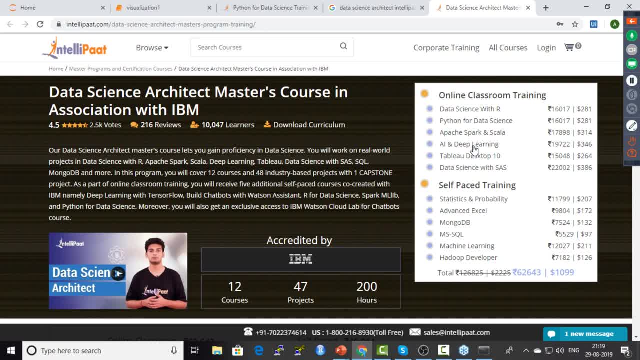 such as convolutional neural network, recurrent neural network and so on, And you'll be implementing all of these different neural networks with Keras, TensorFlow and also TF. Learn right And once you're done with processing the data and analyzing the data, you as a data scientist, 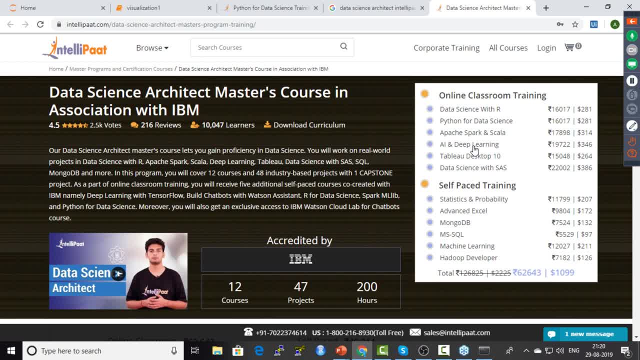 should also be able to represent this data in the form of. you know Python, So that is why we also have this Tableau Desktop 10, right? So with the, you know, when you learn Tableau Desktop 10,, you'll learn how to create stunning. 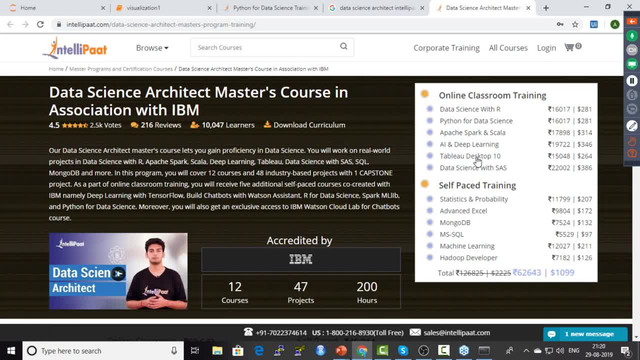 dashboards and you provide these insights to the decision makers, you know, and with the help of those insights they can come up with valuable business ideas. And not just this, you also have this: self-paced courses, self-paced modules, where you learn. 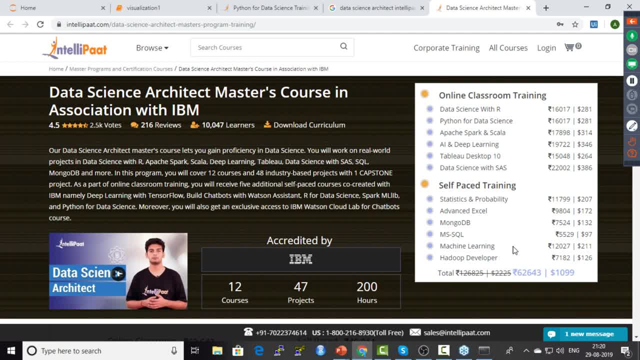 about statistics and probability, advanced Excel, MongoDB, MS SQL, machine learning and so on, And you'll also be able to use this data science architecture course to develop your own data science projects. So if you're a machine learning and Hadoop developer, right. 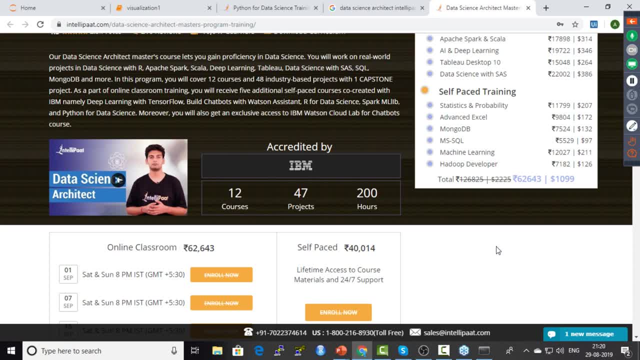 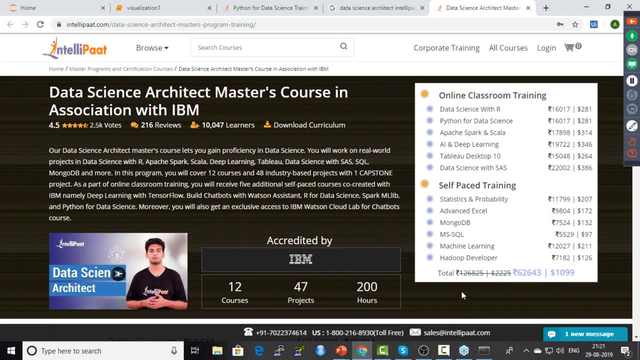 Now one more thing about this data science architect courses. you will have an end-to-end capstone project. So the specialty of this end-to-end capstone project is it'll you know you would need all of the skills which you would have learned from these different 12 modules. 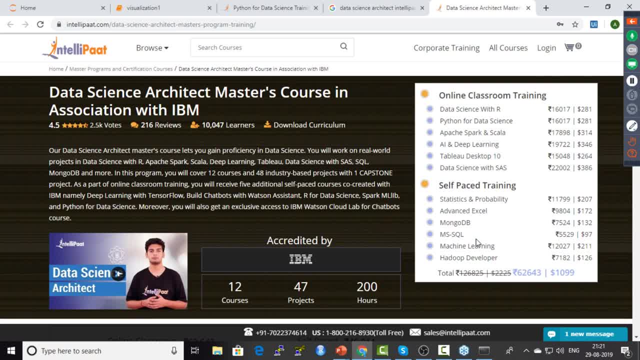 So, using the skills which you've learned from these 12 modules, you would have to solve this capstone project Now. you'll get the certificate by IBM once you complete this capstone project. So that is truly amazing, isn't it Right?